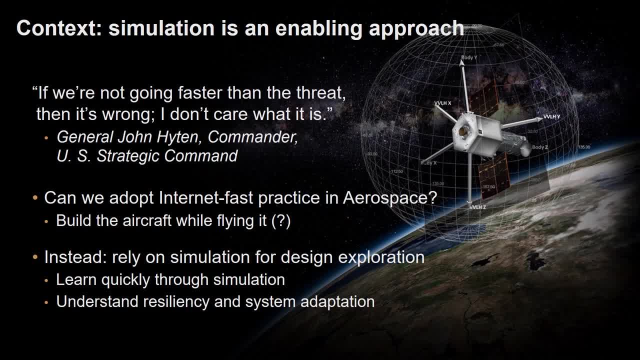 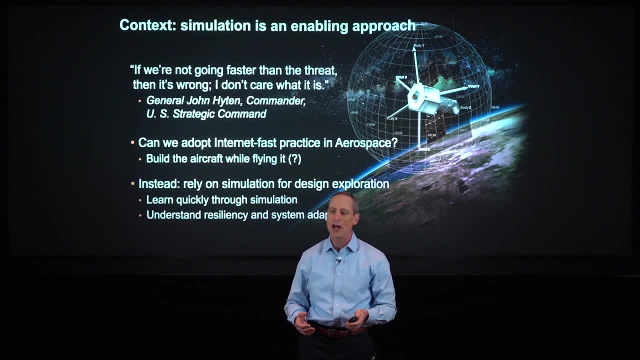 or the service are observing what's happening in the marketplace and adapting on the fly. Every two weeks they come out with a new drop to update the system, And it would be really nice if we could utilize those same concepts for space systems, But unfortunately 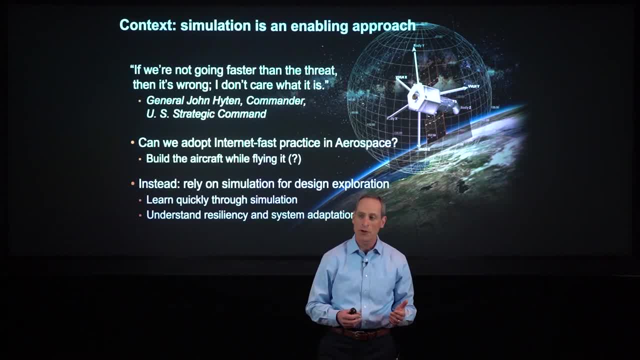 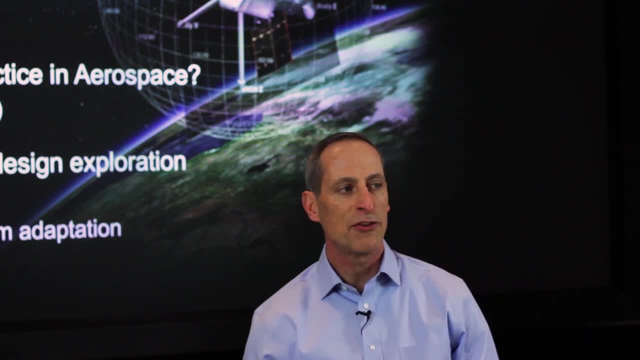 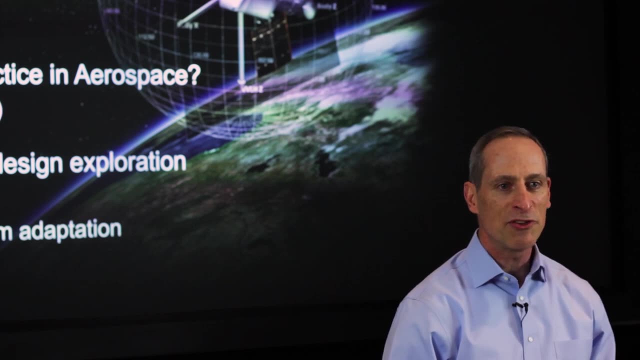 because of the capital investment and the timelines involved. in the physical systems we can't do that exactly, But what we can do is use modeling and simulation to mimic that kind of design. We can build new technologies and new systems in a simulated fashion. We. 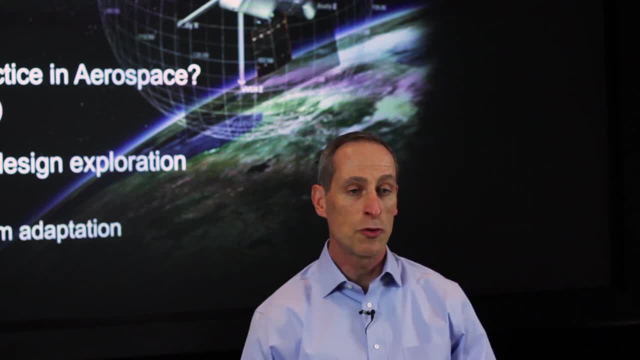 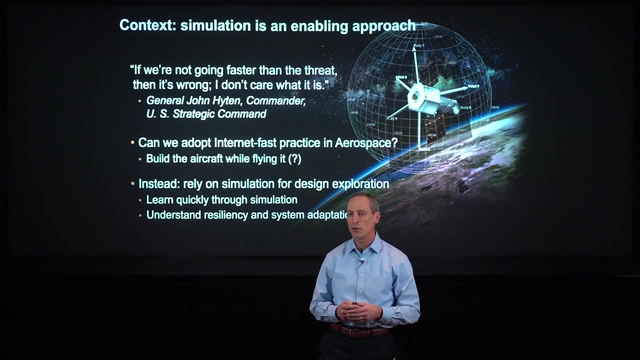 can test them out to provide new services and address problems, And that's what we're going to do. We can address new threats that we might conceive of And we can do that iteration very rapidly. So that's the context for what it is we're going to talk about today. 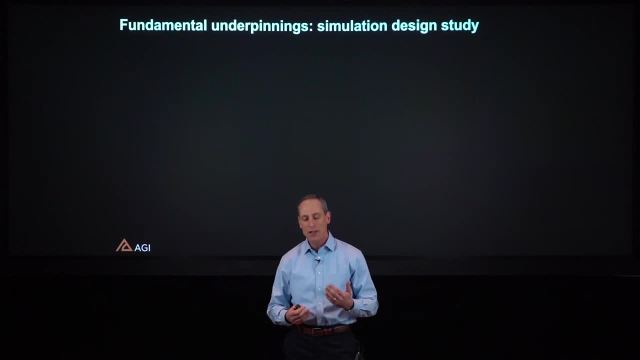 So, in order to achieve new and better outcomes, let's benchmark where we are today. So there are only really a handful of steps that we go through in this modeling and simulation process, And the first is we build the model. So let's assume that process takes us about. 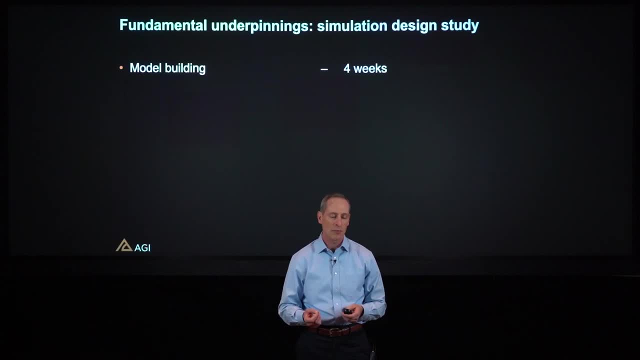 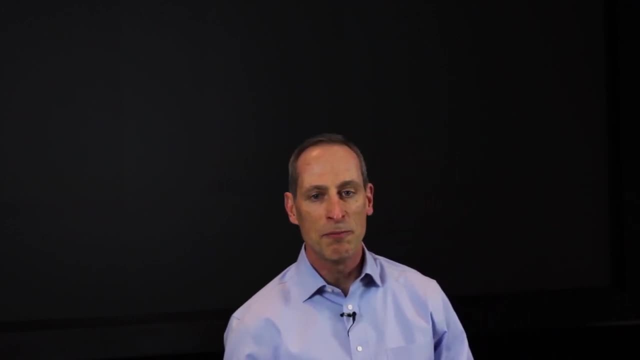 four weeks to build the fundamental underpinning, the point of departure that's going to bring us to where we want to represent our space system architecture. So we've got a couple of orbits, We need a constellation design, some mission payloads, some measures of effectiveness. 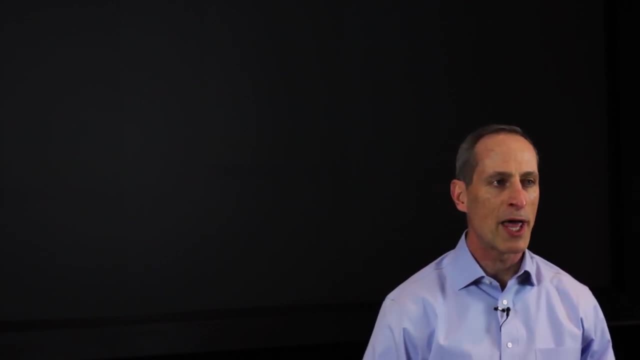 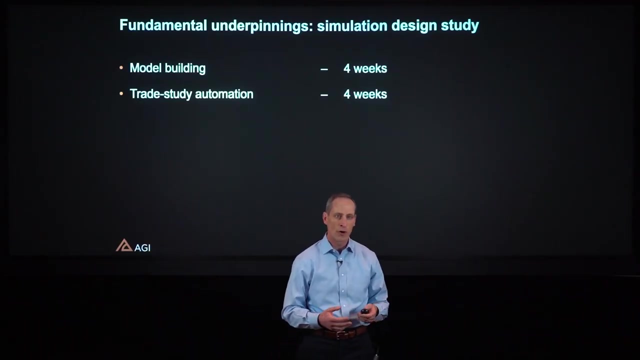 and regions of interest that we care about And that takes us four weeks to build that. Then we have to take that computer model and then we have to instrument it so that we can evaluate it over the control space that we want to consider and look at the measures. 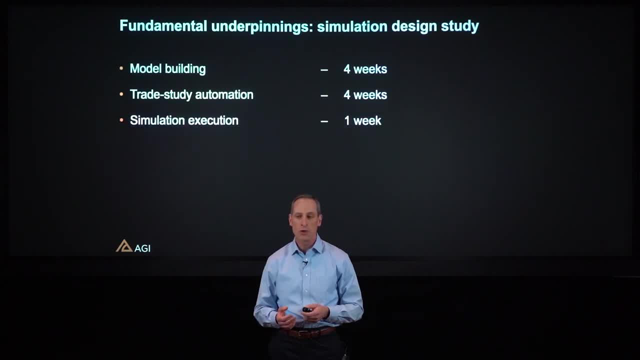 of effectiveness. Now, this is a pretty hefty computer problem, So it's going to take some time to run And it's going to take some time to run And it's going to take some time to run that trade study. So let's assume that the simulation then takes about a week or 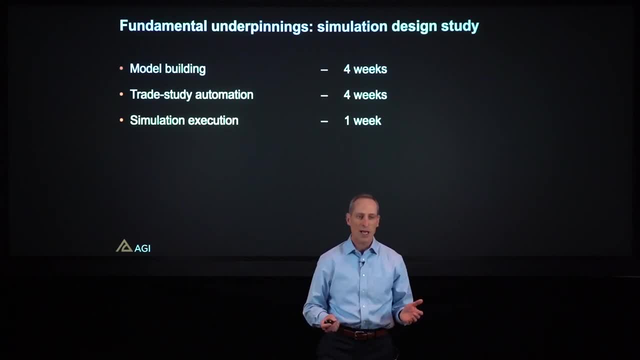 so And then finally we run this calculation and we have this multidimensional output that we then have to analyze and understand. what does all this data mean? So, assuming that takes about four weeks altogether, that took us about 11 weeks to go through that iteration. 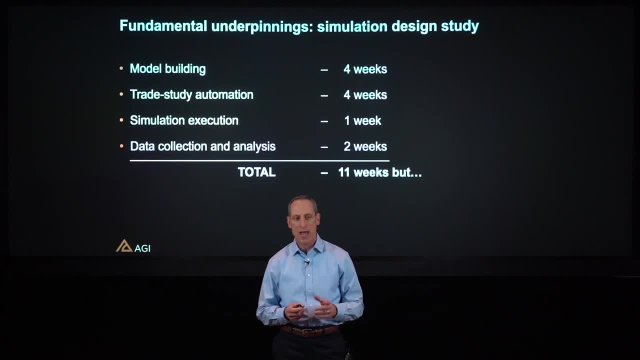 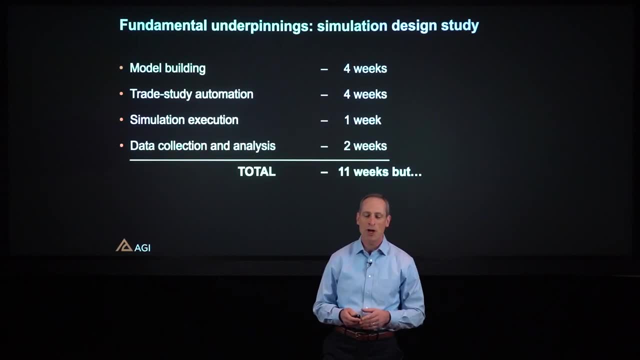 which isn't too bad in the timeframes that we're thinking of, except that that was only our first iteration, And anybody who's been through this process knows that the first time you come through is really just the initial trial, And now you know what you really have. 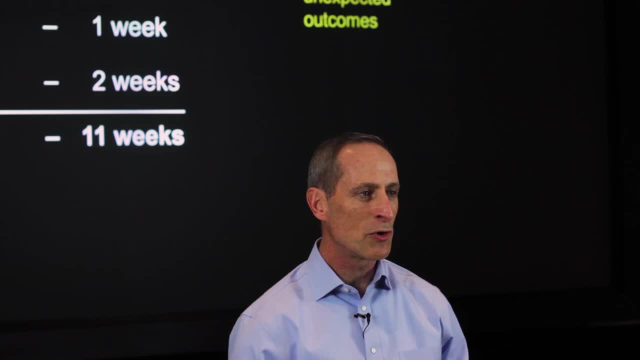 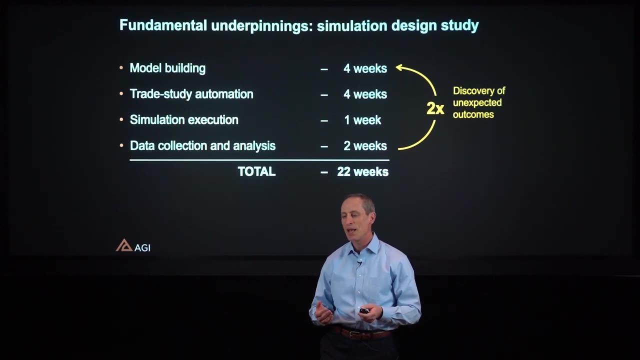 to do So. you discover all of your errors the first time through And you go back and you reset your system And then you go through this 11-week process again, But then, after that 11-week process, what you're going to discover is that there are particular regions. 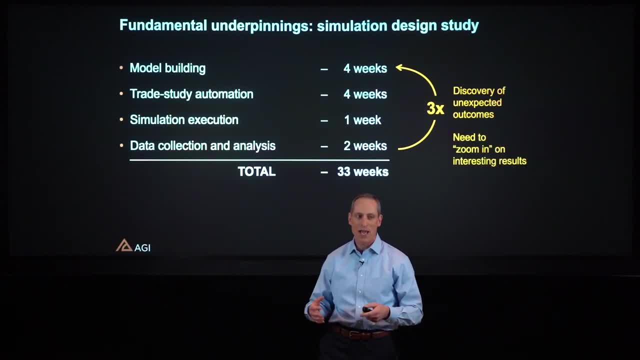 in your control space that you care about more than others. now you're going to zoom in and repeat that process again in those areas, And in the process of doing this, through the first few iterations you made some simplifying assumptions, and now you're getting down to more detailed analysis. 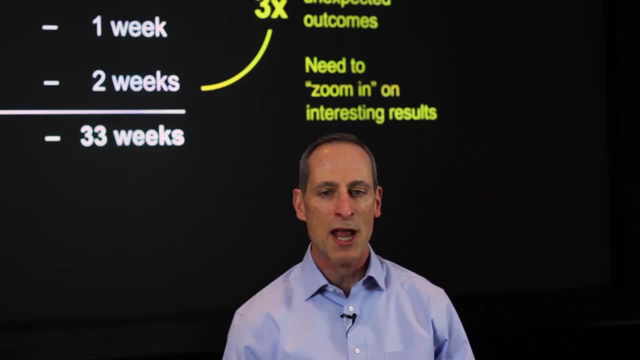 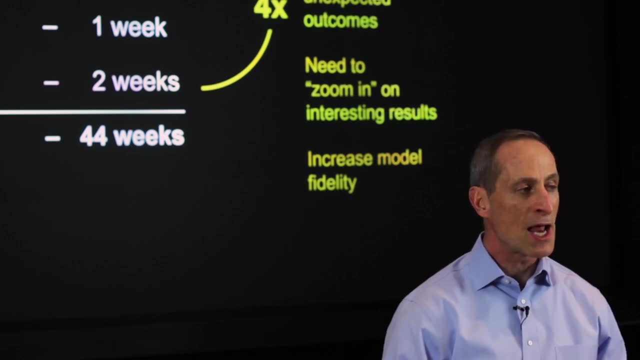 and you're saying: you know what, the simplifying assumptions just aren't accurate enough. I have to add some fidelity to the model. so you go in, you rebuild some models and you do this process again, and now you got something that you can take to your customer- your internal customer, your external customer. 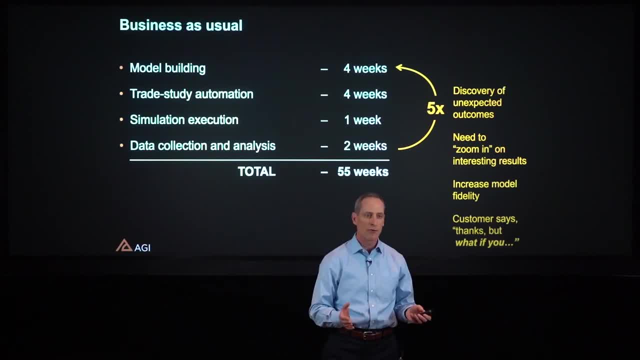 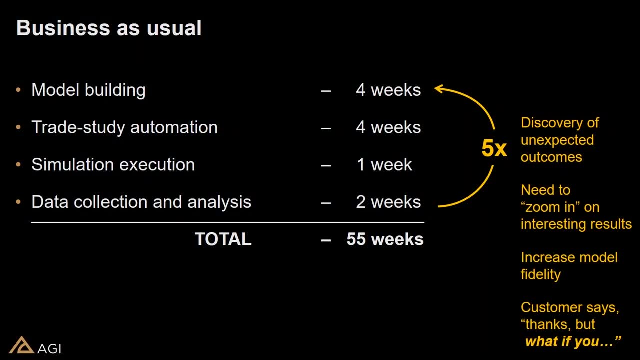 and this always happens without fail, which is, the results are highly appreciated. it provides insights. and now somebody's looking at it from a different perspective and they're saying: you know what? what if you did the following? what if you looked at it this way? and so really just getting to this, 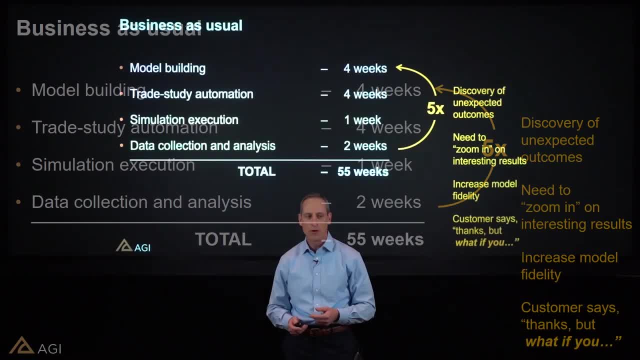 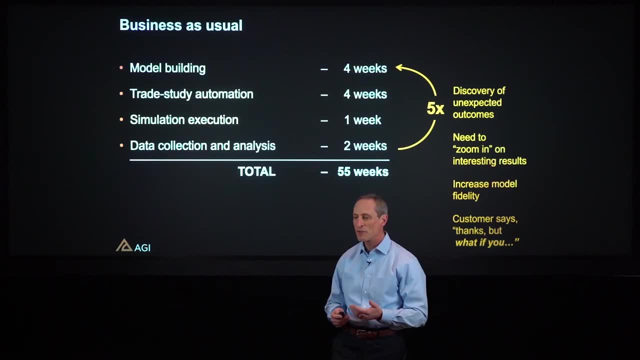 point where you can go back and readdress. the second question took over a year, and that clearly doesn't meet the requirements for what we're trying to accomplish. So what does that mean? we have to do with this fundamental process. Well, we have to take time. 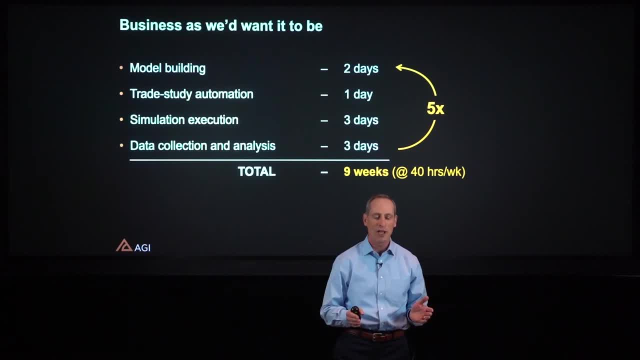 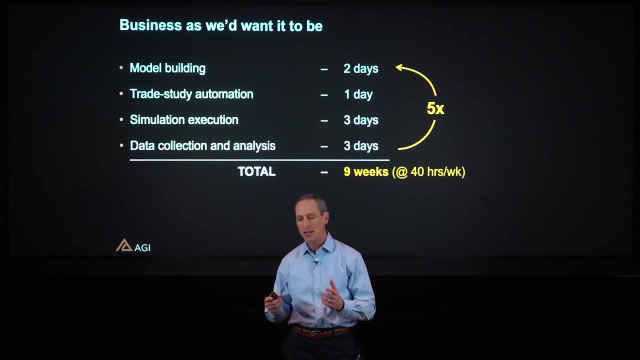 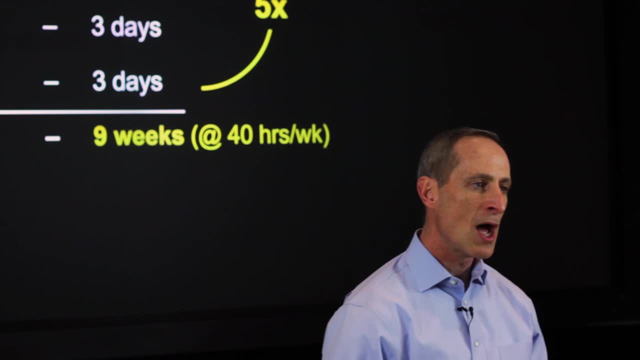 achieve, and we're going to talk about some of the methods that we've learned about in the context of the space system architecture design to make this happen. Before we go on to the specific reference problem, I want to dive into one particular aspect of this, which is the simulation execution time and the 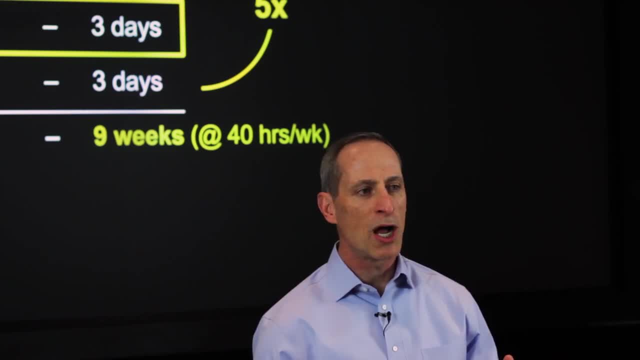 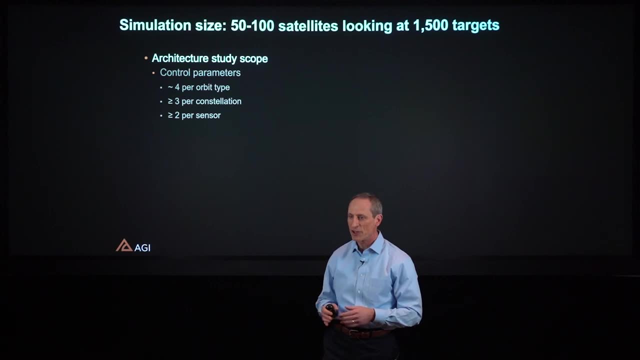 reason I want to do this is because we need to keep in mind the scope of these computational analyses, which can get pretty large. So again, let's break this down into basics. if we whittle this problem down into more or less the smallest number of control parameters that create a viable problem, here we can. 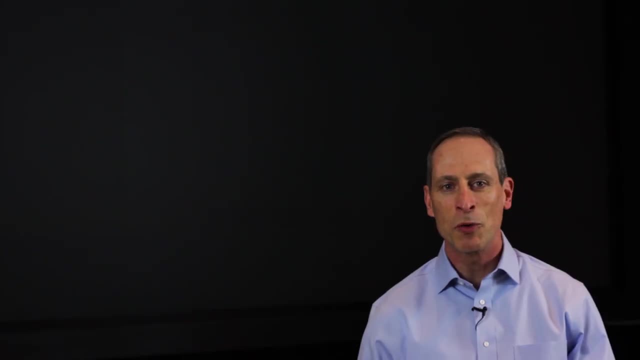 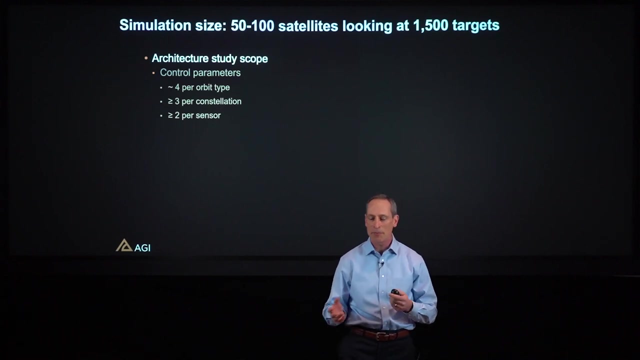 break it down to about nine parameters. so each orbit we can define with at least, well, a minimum, of four parameters, three more to describe the constellation design and for the primary mission payload they're going to be at least two parameters: something related to its geometry, something related to its resolution of 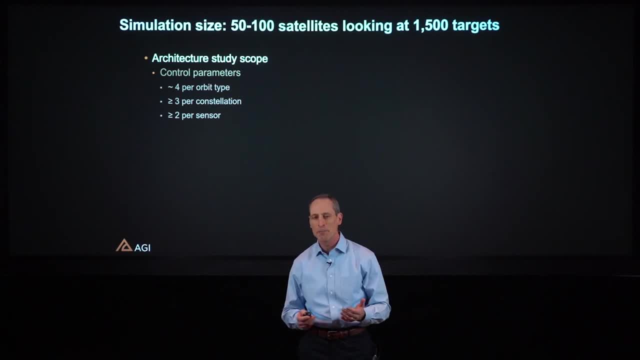 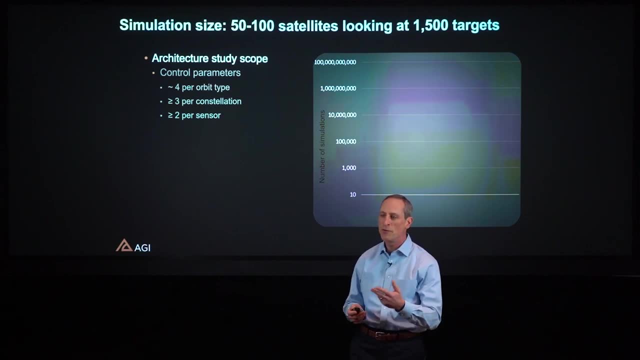 performance quality. so we've got nine parameters. if you just look at the basic parametrics here, if we consider an analysis that only utilizes two values for each of these control parameters and we do a full parametric scan, that's about it is exactly 512 unique simulations. if we now increase the 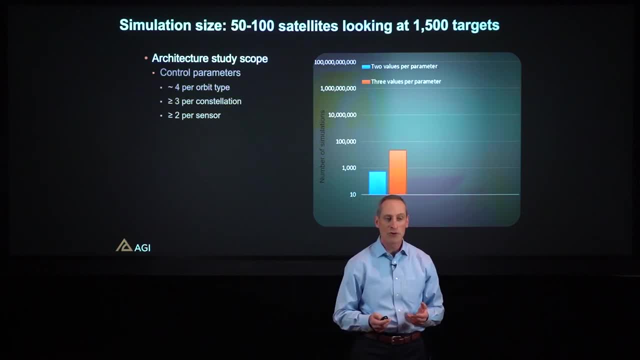 number of unique parameters to three, that number jumps dramatically to 65,000 or more unique simulations, And that's just for the minimum baseline problem that we're considering here. So 65,000 unique simulations to evaluate this trade space through one of those iterations. If you consider increasing 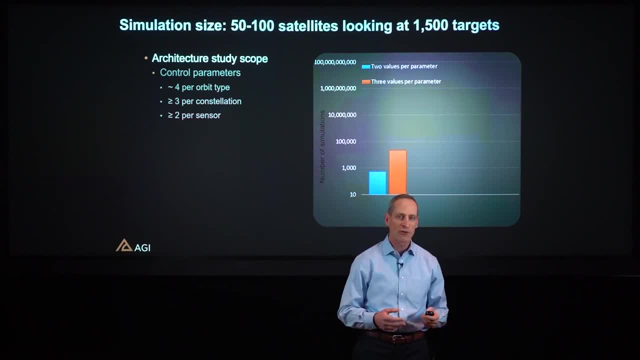 the scope of this. say, your constellation or your design incorporates multiple sub-constellations, two or three. these numbers grow exponentially and recognize that you're looking at a log scale here. So these numbers get very big very quickly And if you look inside any one of these simulations, you find that 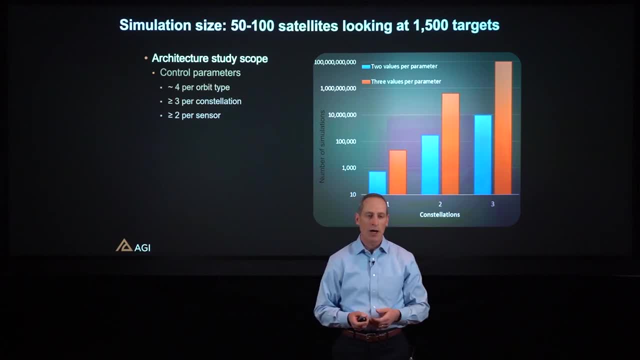 there are a lot of calculations that go on. So for a scenario the kind that we're considering here- between 50 and 100 satellites looking at a distributed set of target points, say 1500, your looking at at least on the order of a hundred thousand unique access. 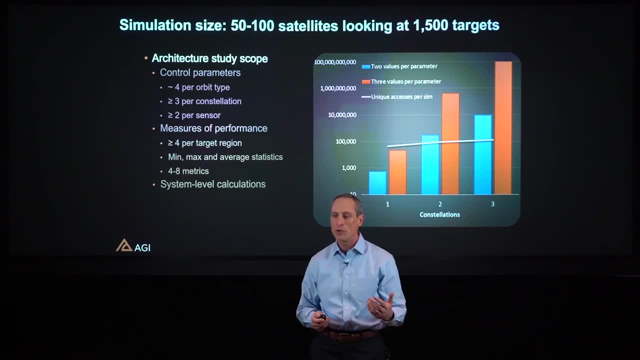 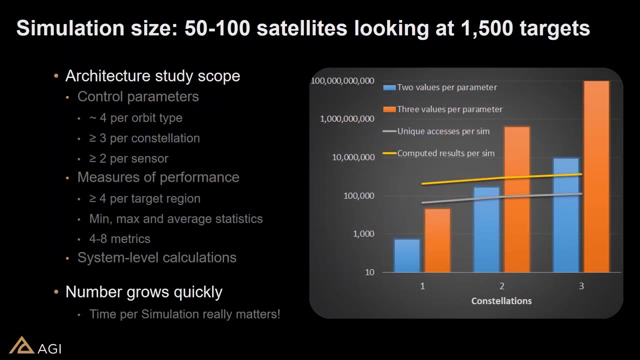 calculations, and then, for each access calculation, you've got multiple measures of effectiveness. so we're going to have eight measures of effectiveness and then, over the simulation period, we're going to calculate several statistical properties. so for each simulation, of which there are hundreds to thousands, there are between half a million and a million unique calculations in the 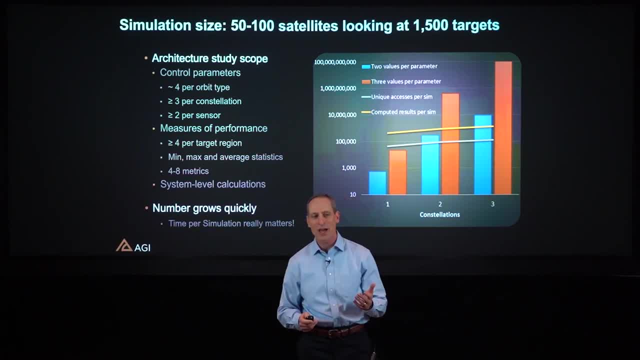 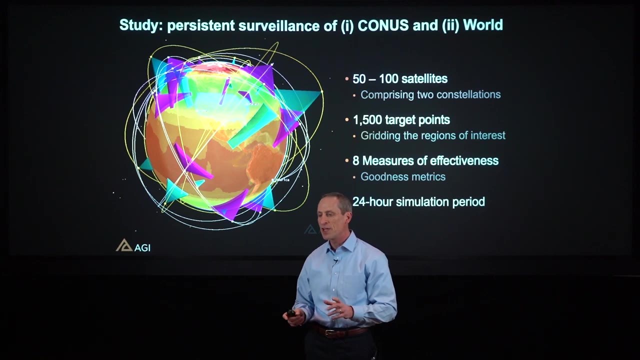 simulation. so I'm just trying to set the mindset, in the context of having to move quickly, that these computations are going to be large and the fundamental calculation engines underneath need to be designed to address this kind of problem and they need to be scalable. so with that as a background, let's get into 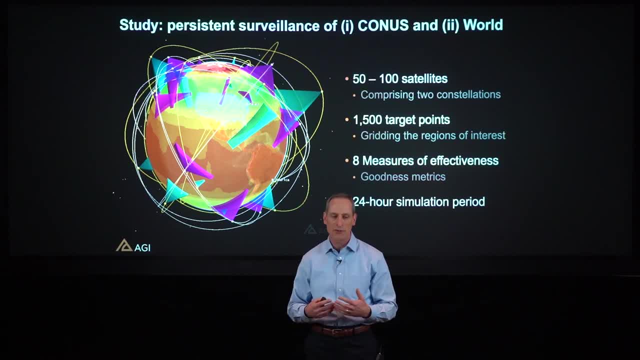 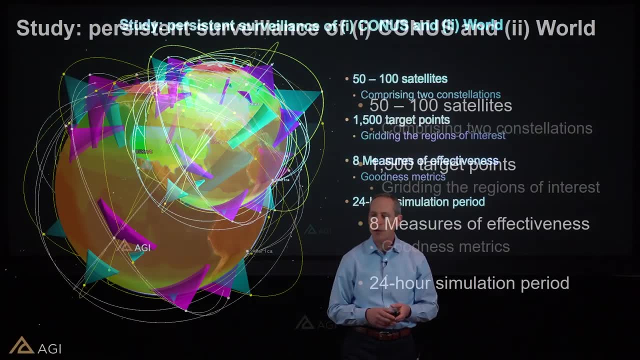 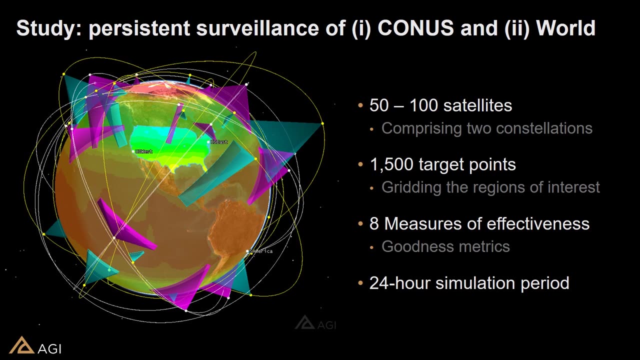 the reference example so that we can talk about some of these things a little bit more tangibly. so here's the reference scenario that we're going to use for this hypothetical architecture study. we're going to look at a persistent surveillance mission and we'll look at a design space composed of somewhere up to a hundred satellites and 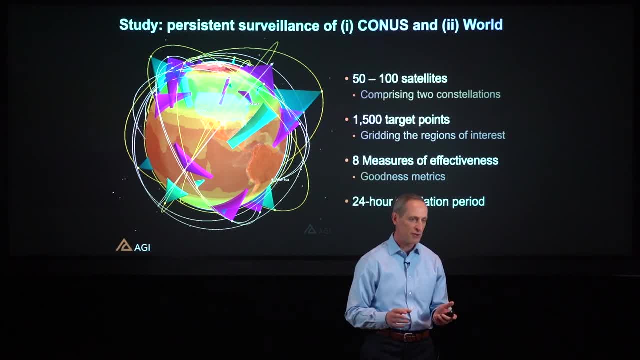 we'll look at two distributed sets of targets over two regions of interest. we'll take a global region of interest and then a higher priority region, just so we can add some interest to this problem and look at some other factors. and for the sake of illustration here we'll say that high priority region is: 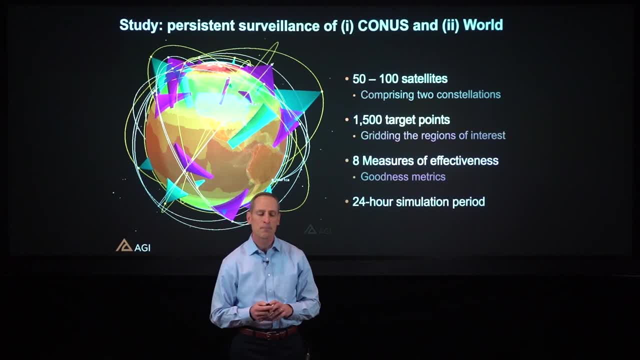 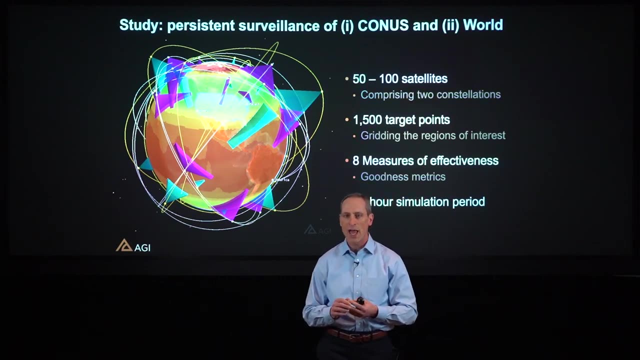 the US United States continental region and then we'll grid those up into about 1,500 grid points and for each of the regions will have four measures of effectiveness: for system response time, for imaging resolution, for time between collections and the number of collections made on each target point. so we've got eight measures of. 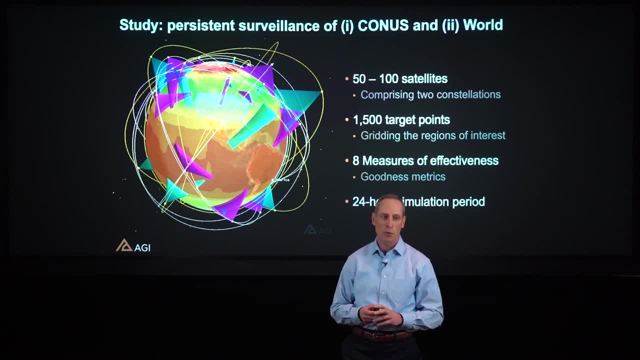 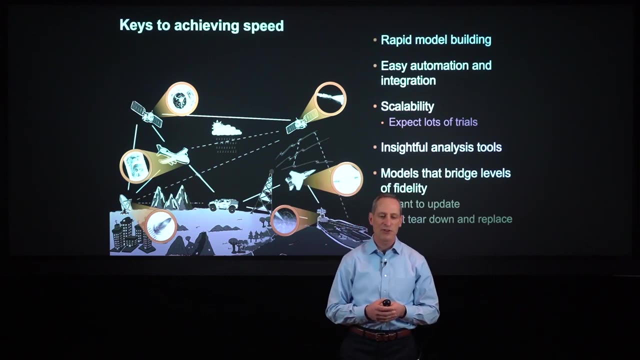 effectiveness over those 1,500 target points and we'll look at a 24-hour simulation period. so that's the scope of the reference example and we're going to go through all those processes that we just talked about in the previous slides to set this up. so in the conduct of our business as a 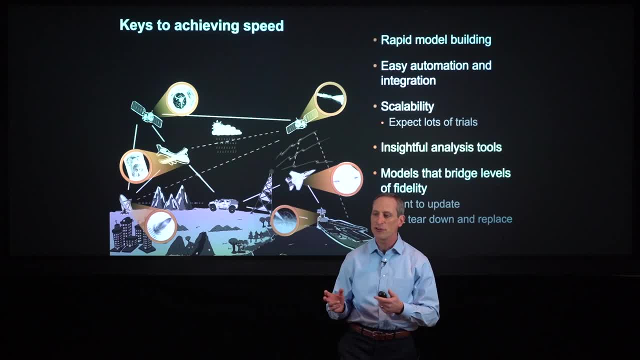 provider of commercial software products to many organizations solving this kind of problem. we've found that there are five key drivers to achieving speed and efficiency as you try to solve these architectural design challenges. the first is the ability to build models rapidly. so that's the first and 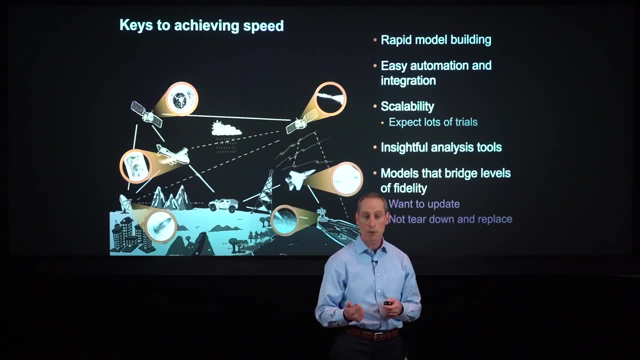 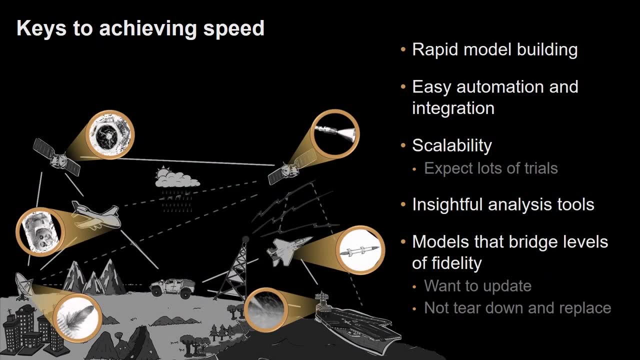 fundamental step is to be able to represent your design concept in a computer model that's executable. that model then needs to be easily instrumented or automated so that it can be evaluated over a range of control parameters and evaluated over all the measures of effectiveness. we spent some time previously talking about how this needs to be scalable, so 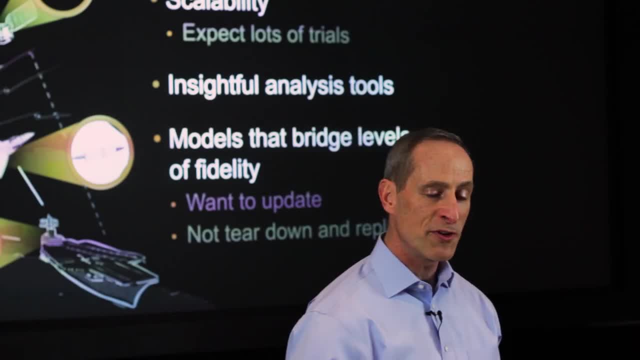 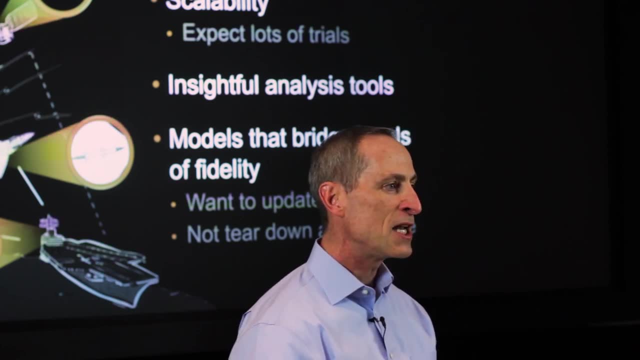 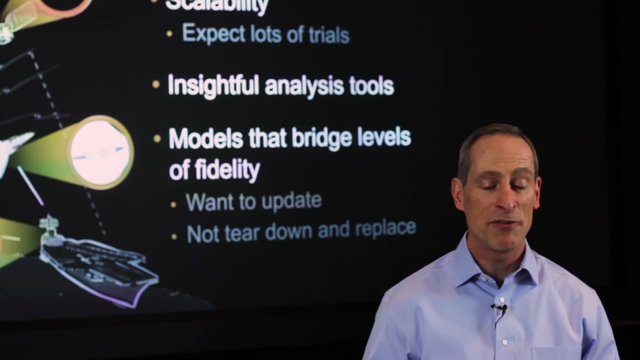 the computational underpinnings here need to operate efficiently for big problems and then ultimately you're going to get a ton of data out of this, looking at many different competing factors, so multi-dimensional data. you need to have tools that take that data very quickly and give you insightful conclusions that you can draw. 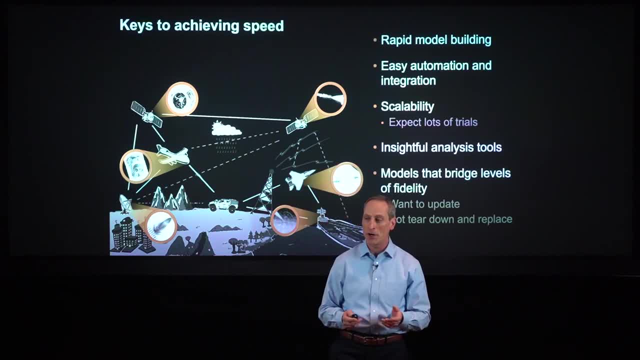 to understand what just happened and where I should go from here, and then, after you complete that process, you're going to gradually go into incorporating higher fidelity models as you look at more and more individual design points. so ultimately, you want to be able to add those level, levels of higher fidelity, or 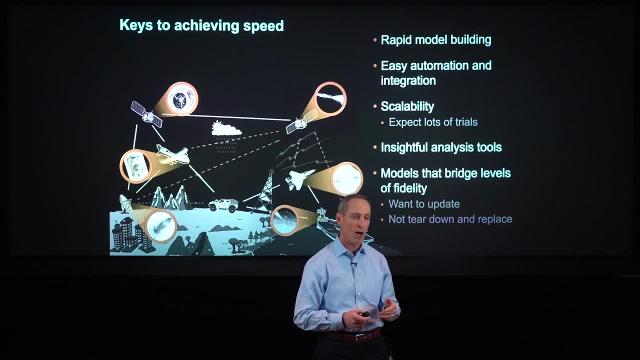 higher fidelity models into that same fundamental mission model, without having to rebuild everything from scratch. so those are the five key points that we're going to emphasize here. we're going to walk through one cycle of that iteration for the first four steps and then I'll talk very quickly about how we 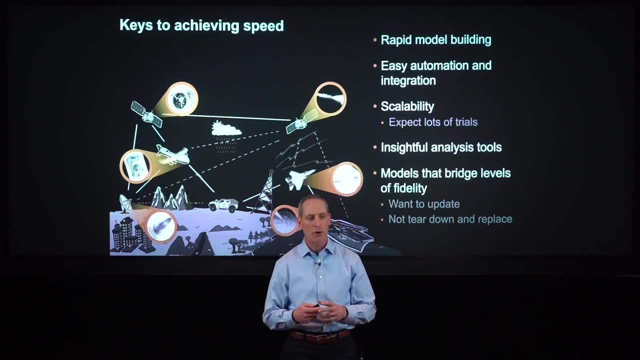 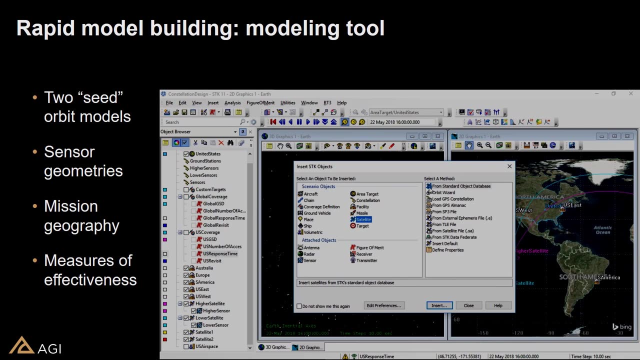 can bridge that fundamental mission model with models that incorporate levels of higher fidelity. so let me talk, start with the rapid building of the mission model. again, we're doing a constellation design here and we need to create our fundamental point of departure. so the first thing to know is that it's always 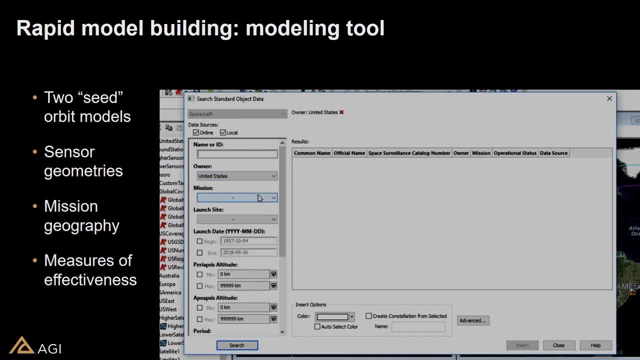 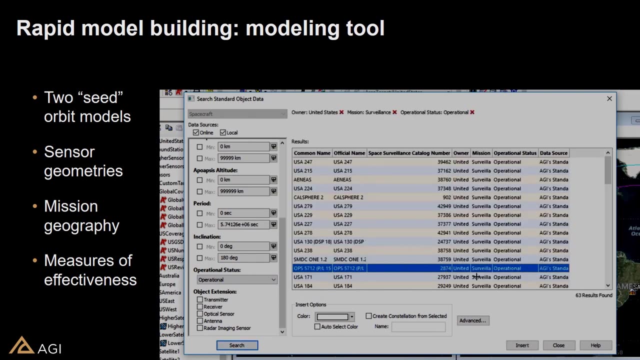 most efficient to start with existing models, wherever they, wherever they exist. so what you see happening here is a look up in a database for existing satellite models that might be good starting points for our orbital design, and these could be models of existing systems or other models that you may have built in. 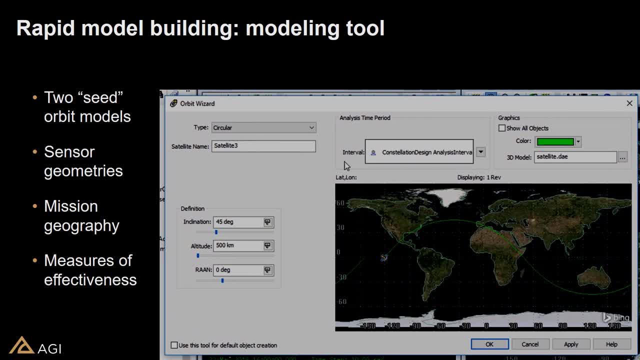 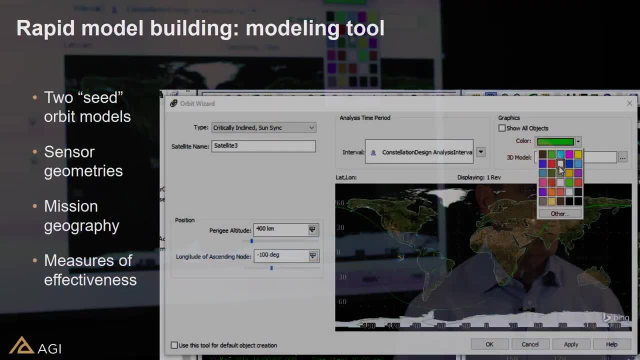 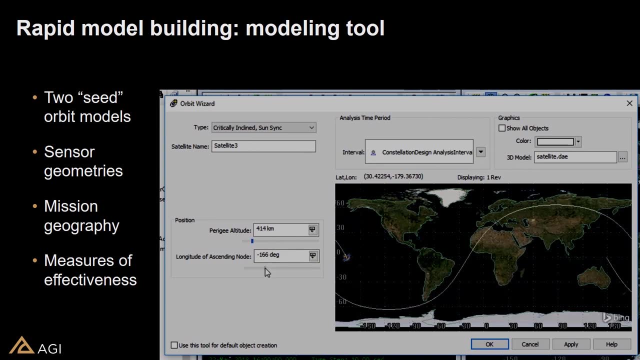 the practice of your business and have just retained. if that's not possible, the most important thing is to get to that starting point quickly. so having tools like this, which are wizard like that, allow you to pick that starting point very efficiently to get that process started, are the next best option. if you're not available, if you 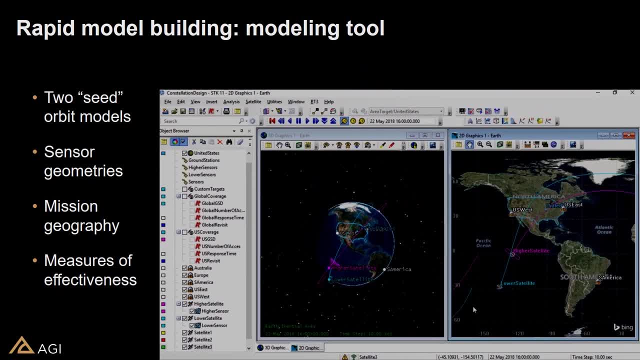 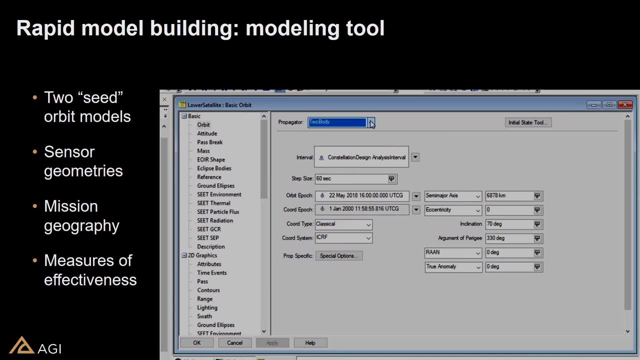 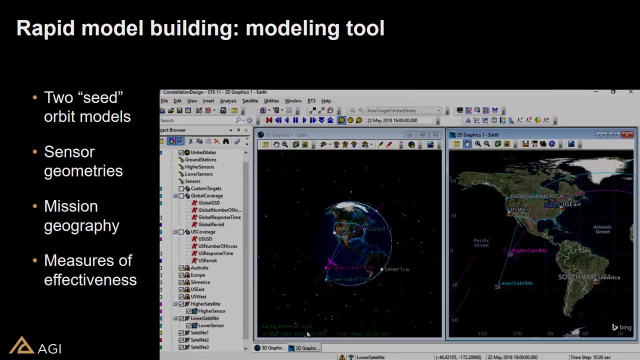 don't have the ability to draw from an existing database once those models are in place. an absolute critical aspect is that all these models are data-driven, that is, all of the finding parameters are available for variation as you go through the trade study analysis which is being shown by this property panel here, then after. 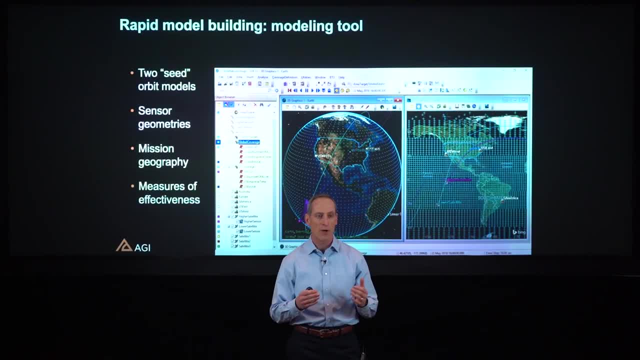 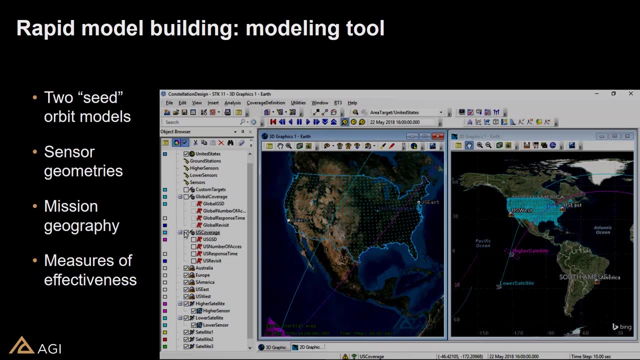 creating the system definition, it's really important to be able to add your measures of mission effectiveness and in our case, these are distributed measures, so you see simple gridding tools that allow you to create the grids over all your regions of interest: the global region, a US region, a region of selected. 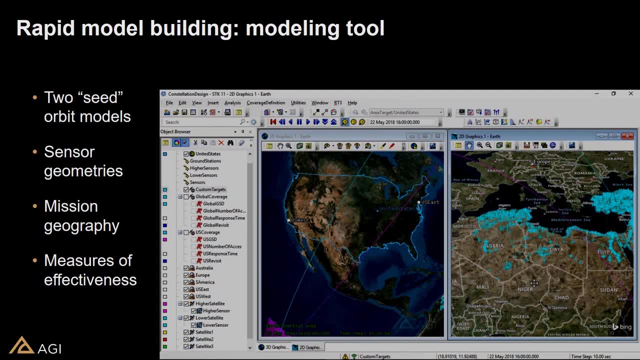 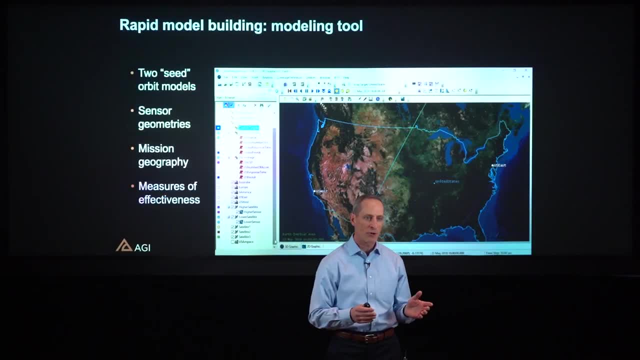 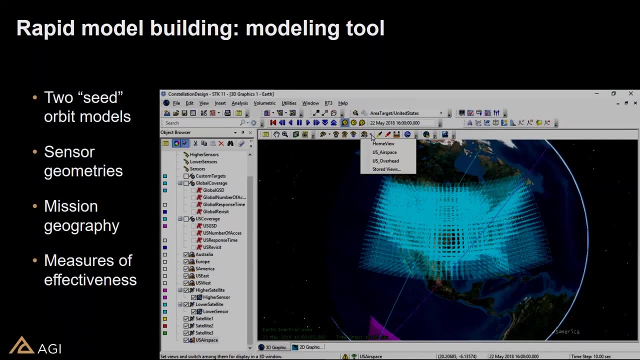 points that you see here, and these, in order to be as applicable as possible, have to be defined in the most flexible way, which means they can't just be points on the ground or constrained geometrically in any way. so what you see being illustrated here is the ability to do that same type of gridding very 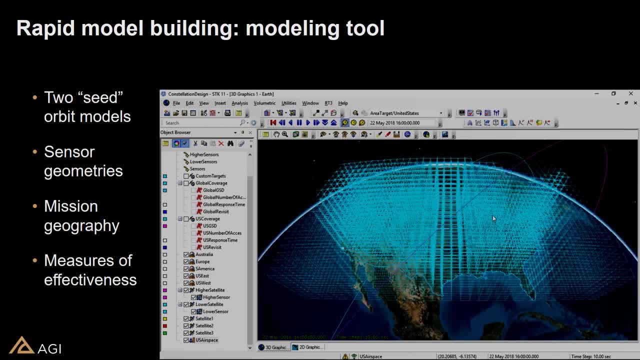 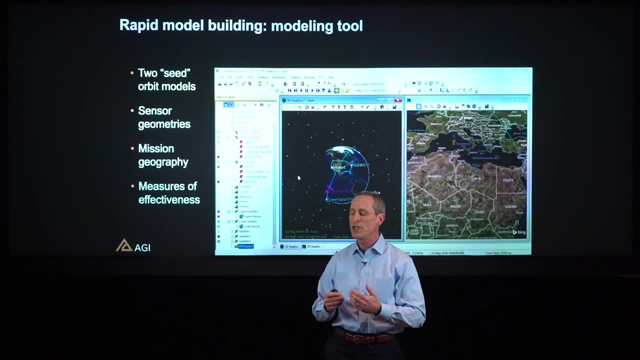 rapidly over a distributed region through space, in the airspace, on the ground and in any dimension. and then, finally, for each of these grids, you have the ability to create a grid that allows you. to each of those grid points we have to add measures of mission effectiveness. so 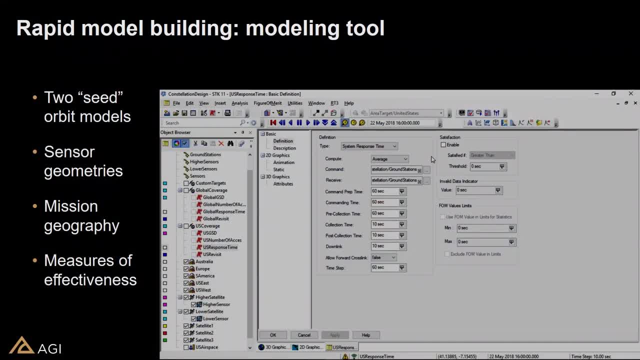 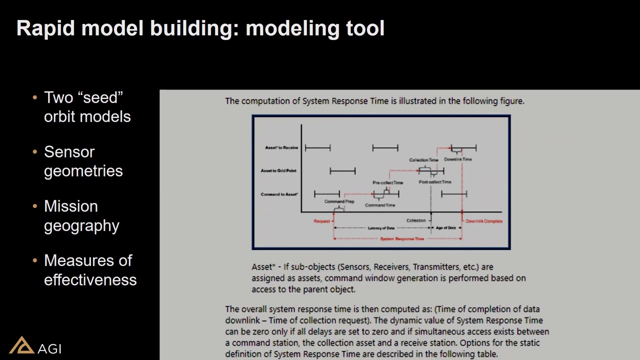 again, the first and foremost criterion is to have your most important measures of effectiveness already available to you in some way. this is one that I like to point out early on in the process, which is the system response time. it's a good starting point that incorporates a lot of good engineering assumptions. so 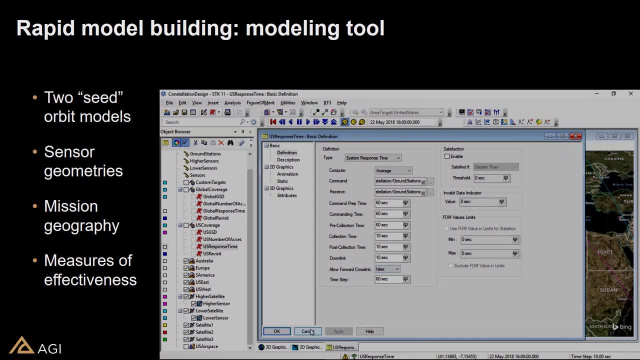 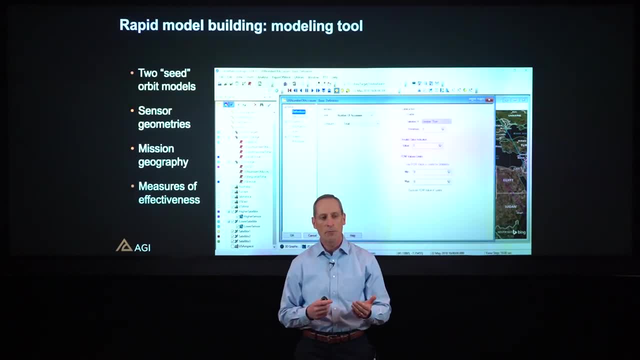 you can do good first-order analysis and then replace this model later on with models of higher performance, and then you can start to create a grid that has a higher fidelity, as you want to dig into each of those parameters a little more closely. ultimately, you want to ensure also that you can include any 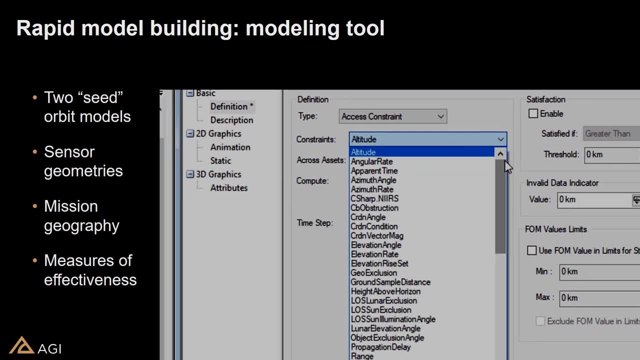 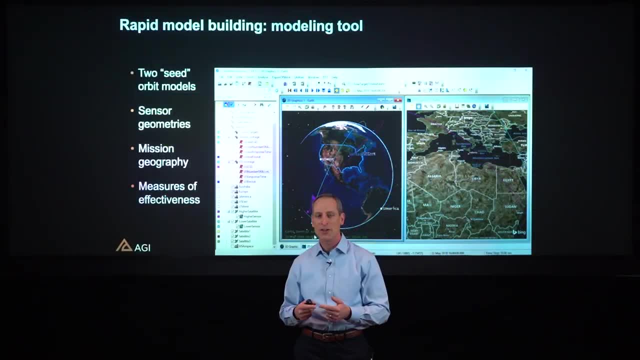 type of model. so the ability to have models that you build that represent your special sauce in your business and incorporate them in a co simulation fashion in this type of simulation engine is also critical, so that you know that you have the expandability, extensibility to do any type of measure. 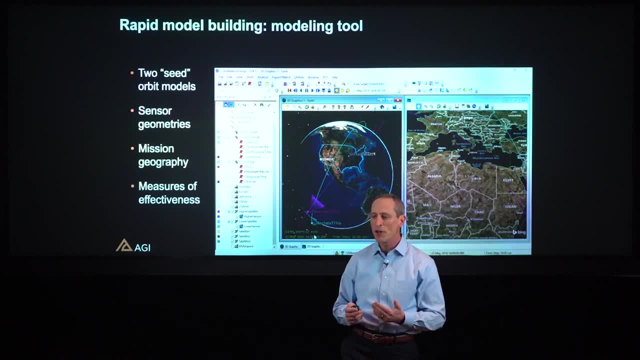 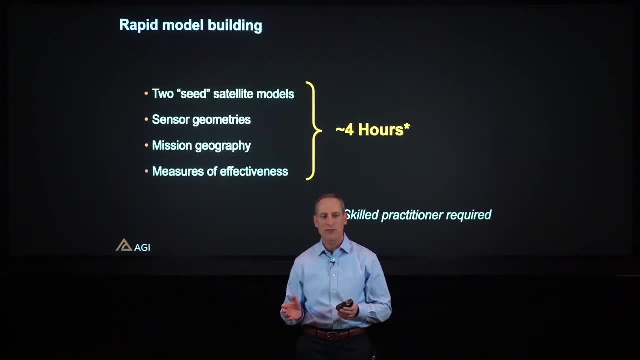 of mission effectiveness that you might need to have in order to be able to do any type of measure of mission effectiveness that you might need to need. so those are some of the fundamental aspects that go into the tools to build those models and when we did this process for this reference. 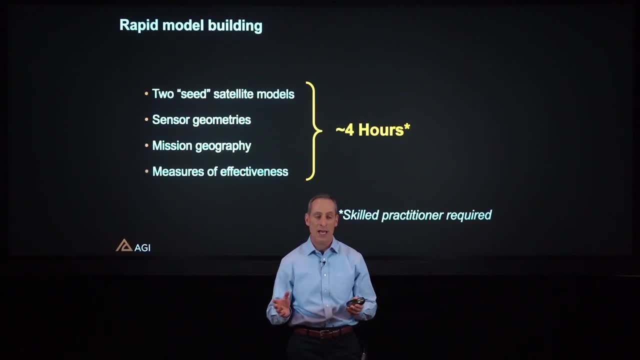 example, it took us about four hours to go through this process, and again that entailed the following steps: we built two orbital designs that represent seed satellites for our constellation designs. we define the sensor geometries. we built the mission geography using those gritting tools that we illustrated here. 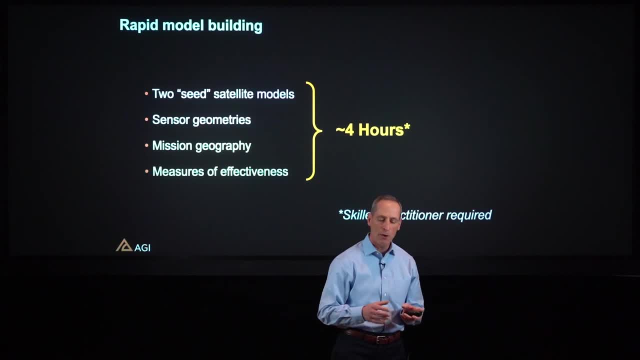 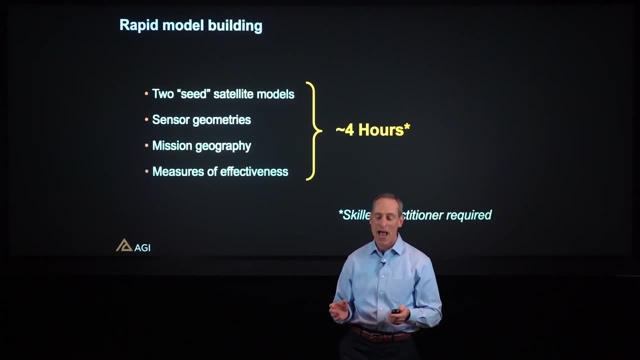 this area. so and other question that needs to be asked when you get around to evaluating- can we do this process quickly and efficiently- is: how quickly can I change, train my staff, my engineers, to use the tools that you're utilizing here? so that is a question that needs to go along with the tools themselves. but 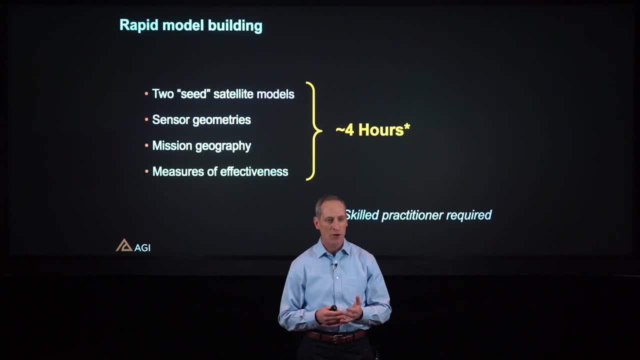 But in general, this type of tool can be learned rapidly and used to create a model like this in the span of about four hours, not four weeks, All right. so the next step, then, is to instrument this model so that we can do the trade study analysis. 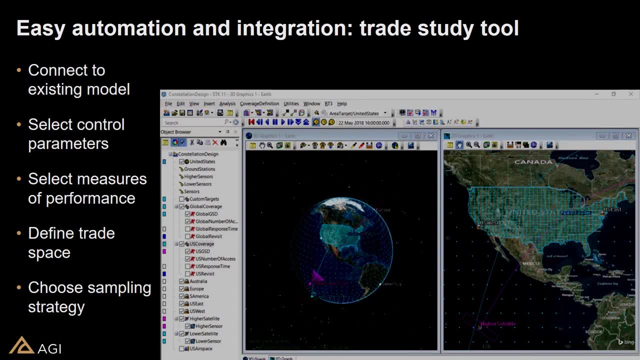 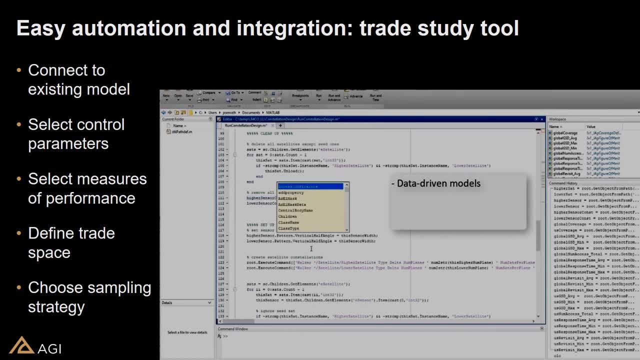 And again, what we wanna do here is connect to those control parameters. We wanna set up the scope of the variation, and then we wanna automate the design process. So one thing that's important is that your model subscribe to open standards that can be utilized. 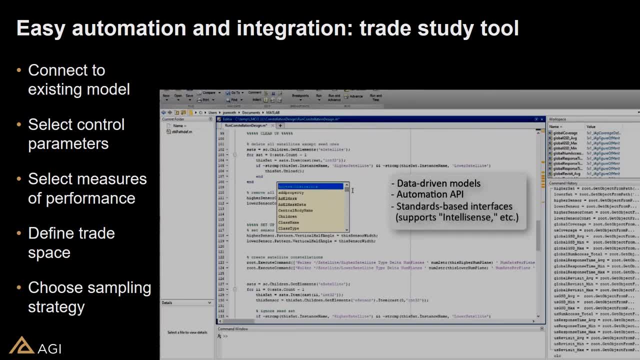 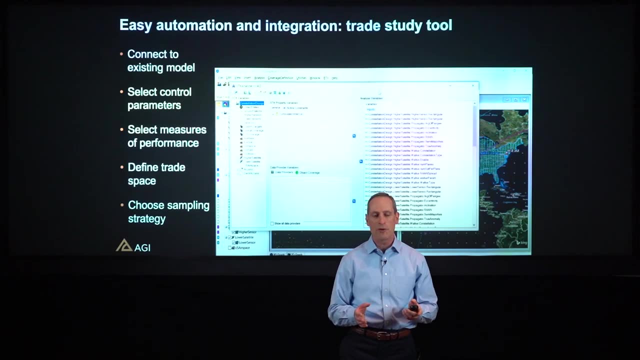 in any tool that you might want to use. So what you see here is a MATLAB environment being used to connect to those control parameters, taking advantage of IntelliSense, so that just about any engineer familiar with MATLAB can automate this type of system. However, if you don't want to do this through scripting, 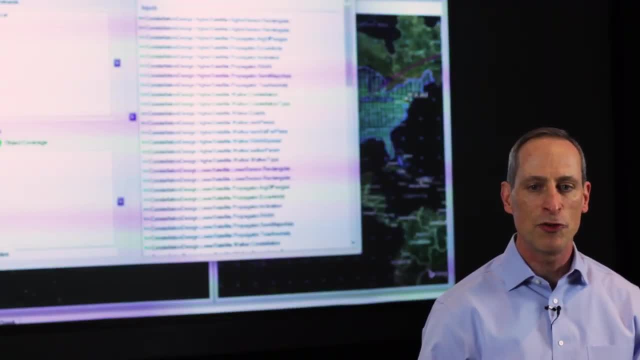 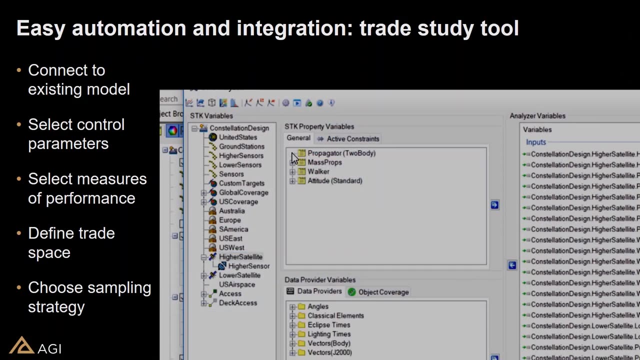 what you can also use are tools that are automatically connected to the mission model. So in this case, what you're going to see is something like a drag and drop environment. So you see on the left panel all of our simulation entities, which are the sources for our parametric variation available. 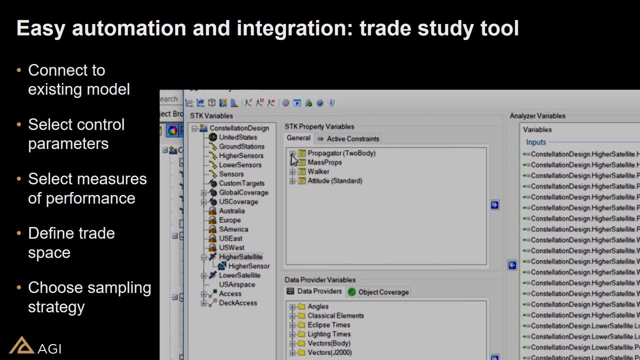 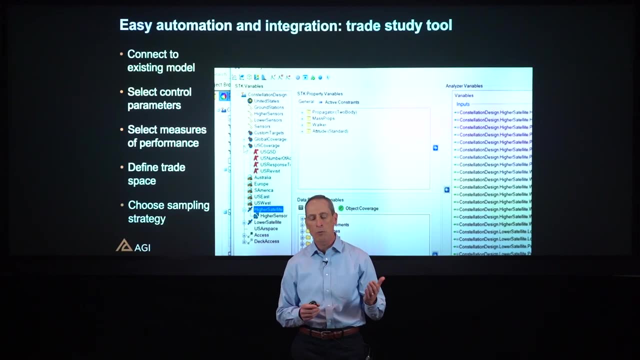 And as you click on any one, all of the control parameters are exposed. So now somebody without any scripting experience can identify what those control parameters are and bring them into the design space, And that applies to the vehicles, the sensors and the constellation designs as well. 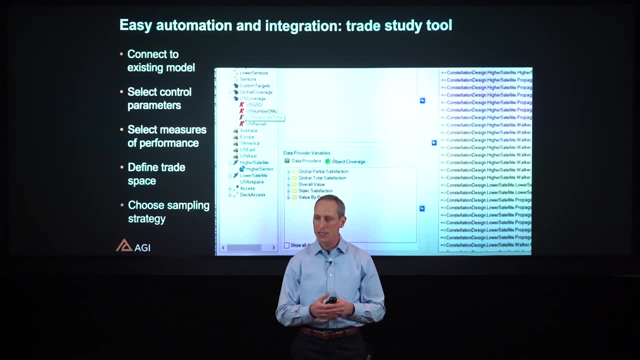 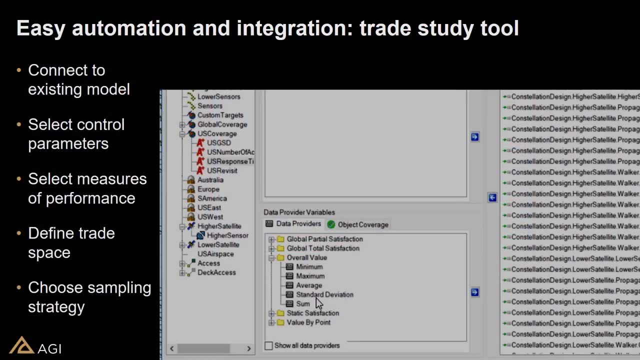 And we wanna do the same sort of thing for the measures of mission effectiveness. So here you see the gridded regions and we can pick the parameters and the measures of effectiveness that we care about. You see that you have options to look at the statistical outputs. 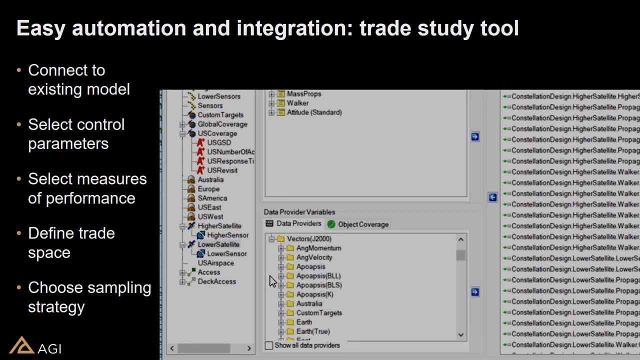 for each of these that you like. And again, it's a simple point and click, drag and drop: creation of the trade space. And really what we're doing here is just identifying the scope of the parametric variation for our trade study analysis. 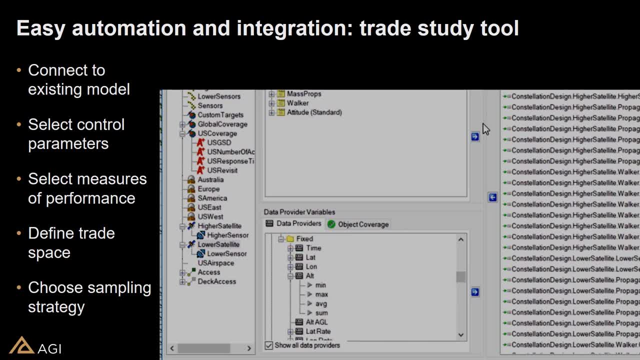 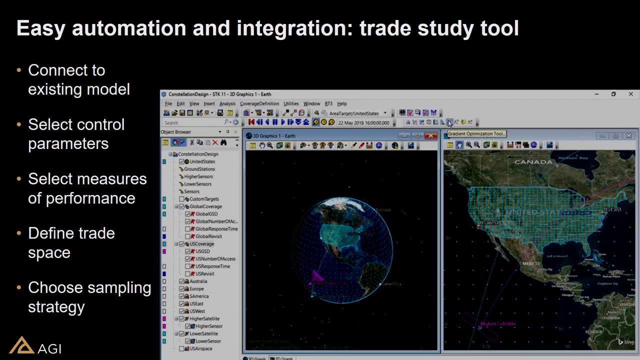 What you see illustrated here is the depth to which you would like to be able to go for each of these parameters. So if I cared about the altitude constraints on an individual satellite, I can go to that level of detail. With that defined, the next thing we need to do. 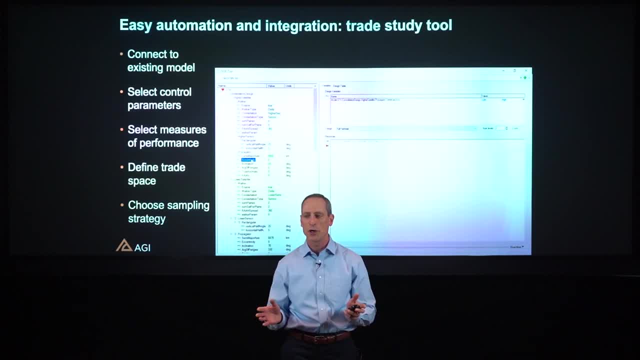 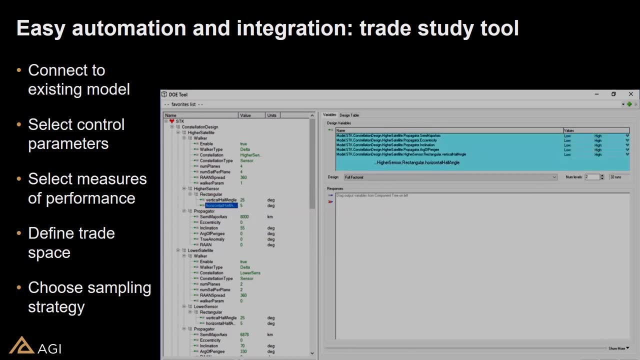 is define what the scope or range of the variation is going to be, And this can actually be, at this point, a different engineer from the constellation designer. So they're actually bringing in the control parameters here and now we're defining what the bounds on that variation are. 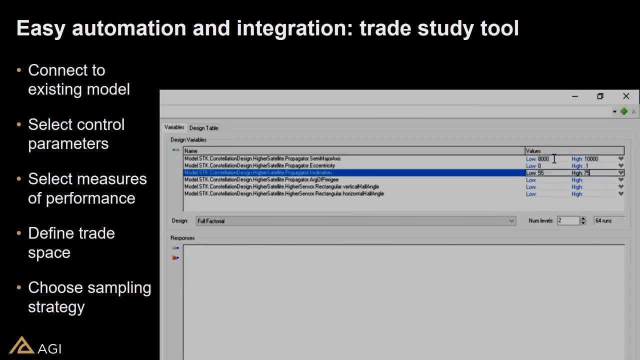 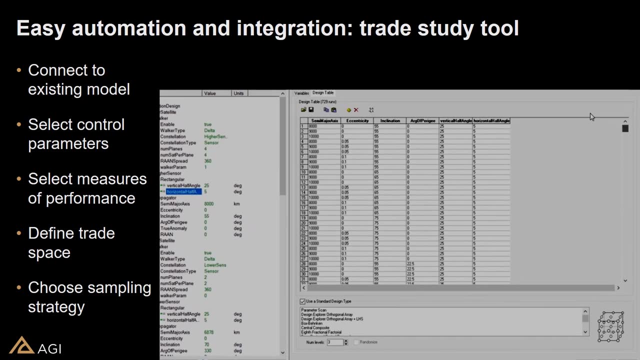 So that a system engineer, without explicit knowledge of the details of the system, can safely run these trade studies without violating any fundamental constraints. You'll see here, if we do a full parametric scan and you're looking closely at the number of iterations, it's somewhere over 700.. 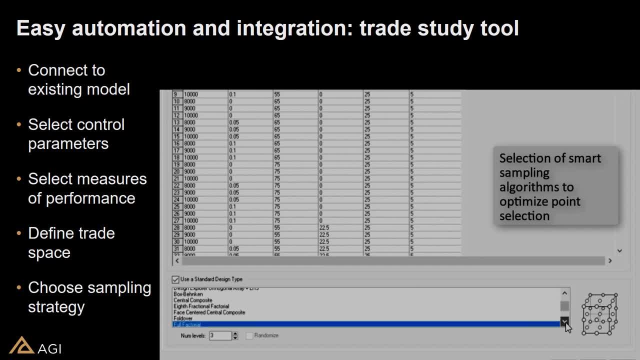 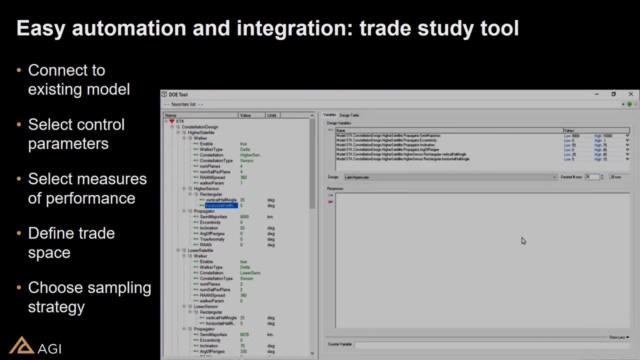 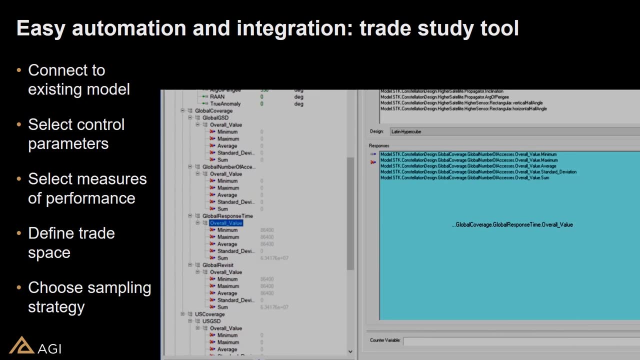 Another important thing is to have integrated smart sampling parameters. Parametric scans in general for continuous variables are not necessary and a pretty inefficient way to do things. So, if you paid attention, we reduced the number of iterations there through the sampling algorithm from more than 700. 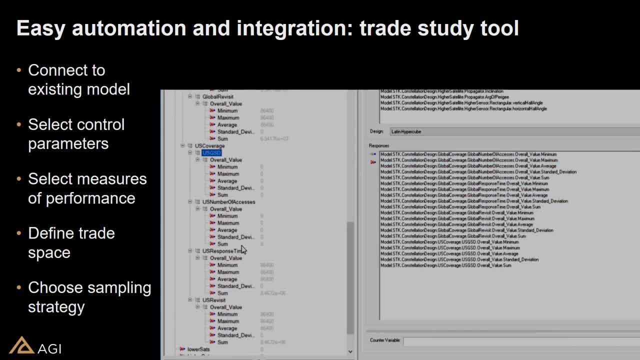 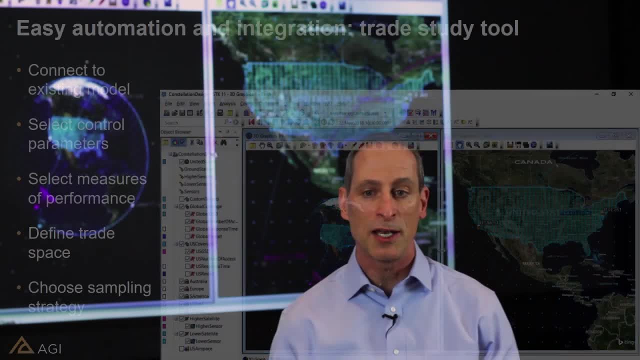 to fewer than 30, which is a great time savings. And now what we're doing is we're bringing in all of the different measures of mission effectiveness and then we have our trade study fully designed. The final step is to ensure that this kind of tool. 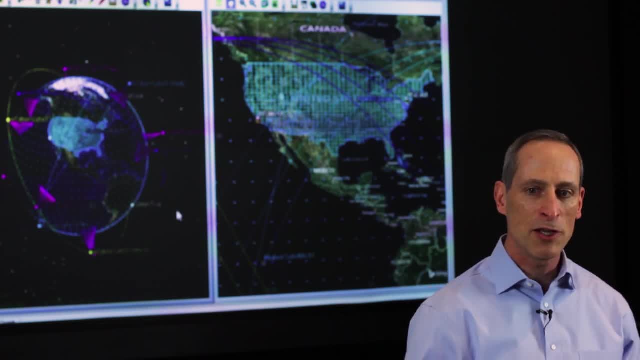 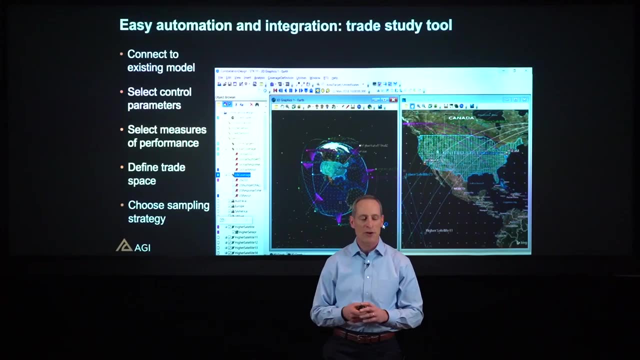 connects automatically to your mission model so that you can, without any other scripting or interface machinations, just run that trade study And what you see happening here is the mission model being executed in an automated fashion through the first iteration of that trade study to create the constellation from the seed satellites. 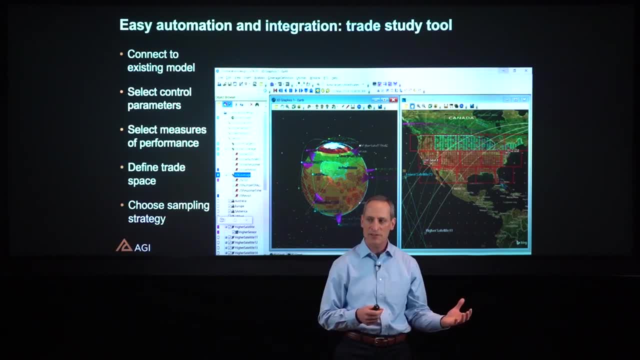 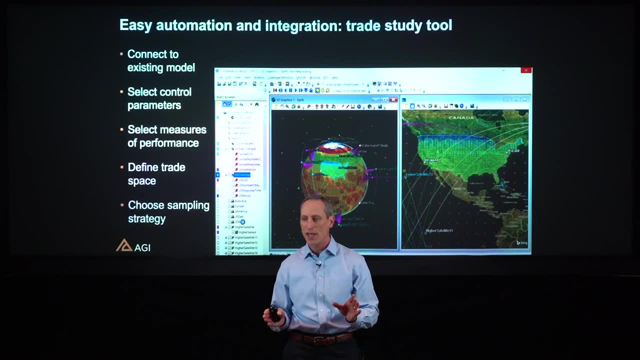 to apply the sensor geometries that were defined in that trade space evaluation and then to perform the calculation of the measures of mission effectiveness over the global region of interest and the US region of interest. So, again, this is just a rapid walkthrough Of the fundamental things that are required. 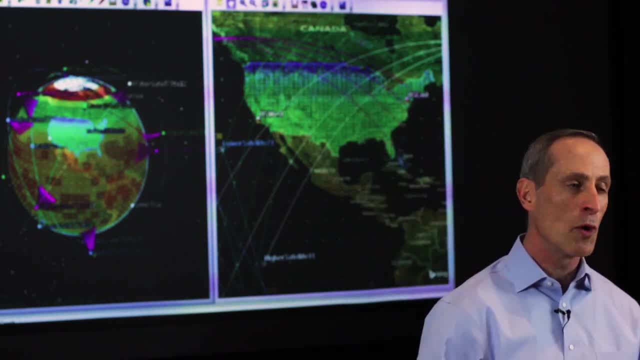 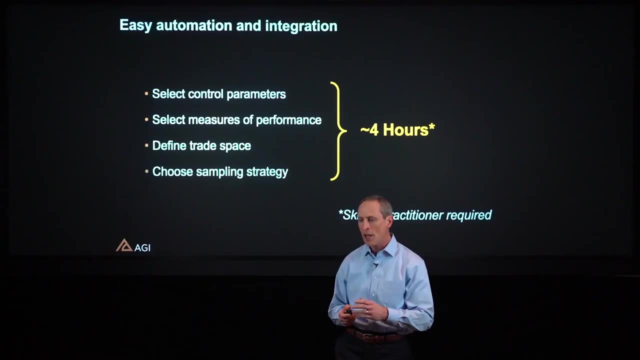 in order to automate a model and execute a trade study. And again, what we're focusing on here is doing this quickly, Setting it up quickly and making sure that it can execute efficiently. When we did this for this reference case, this took us about four hours as well. 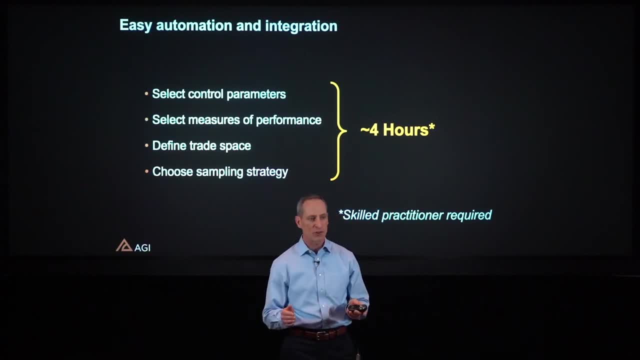 So in the span of a business day we were able to create the mission model. we were able to define the trade space and run the first iteration of that trade study So well, instead of just motivating people. so we then were able to actually apply for residence. 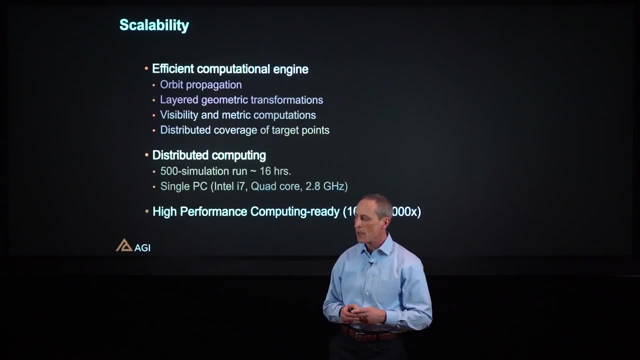 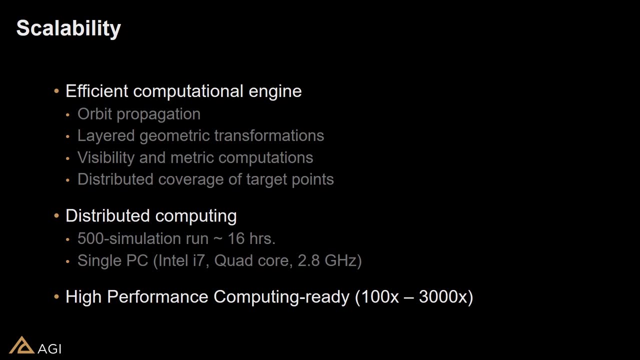 and launch the trade study within that first iteration of the trade space analysis. So now let's talk about the execution of the trade study. So there are several things that are really important in the execution. First of all, the tools that you're using. 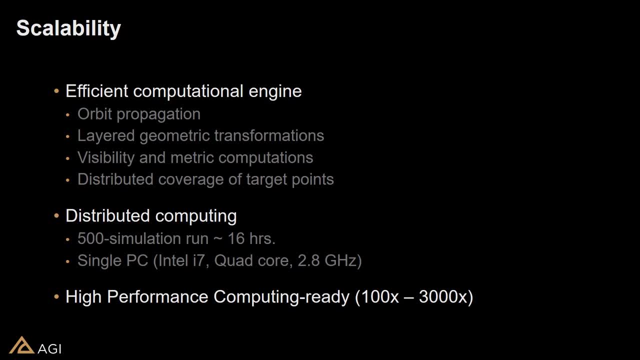 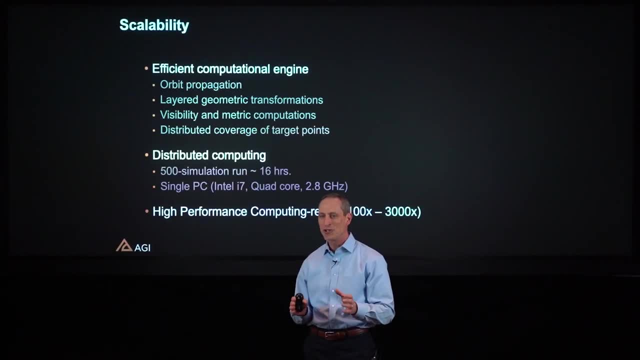 need to be designed to solve the kind of problem that you're looking at. There's no getting around trying to fit a square peg in a round hole. So if you are trying to force fit a tool to do a job, going to pay the price, and these kinds of problems are significant enough that 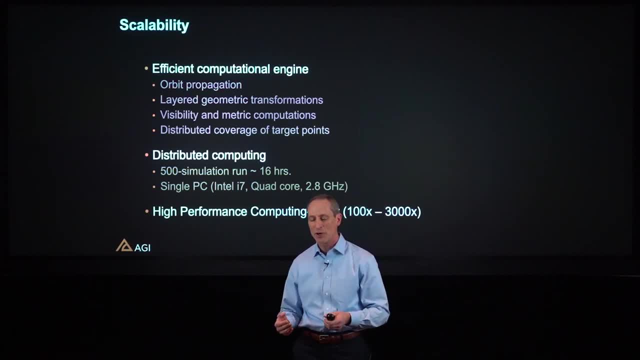 you'll see that issue right away. So in our case, we chose a computational engine that was designed from the ground up to solve these kind of problems, that incorporate the ability to rapidly propagate orbits, layer all of the geometric geometrical transformation, do the gridded calculations and applied. 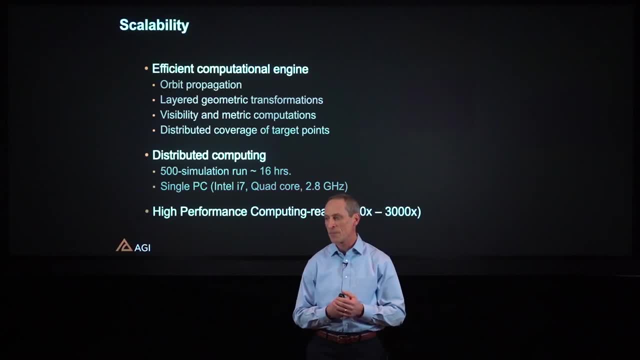 layered constraints so that we can calculate measures of mission effectiveness. Additionally, because of the scale of the problem, we want to ensure that we can take advantage of computational resources, so we want to ensure that we can utilize distributed computing wherever it makes sense. When we ran this, we just used a single engineering grade laptop computer and 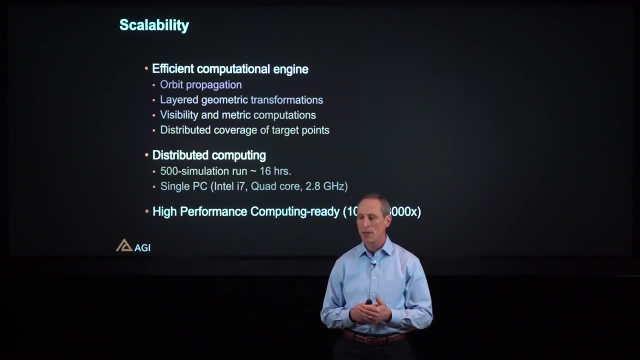 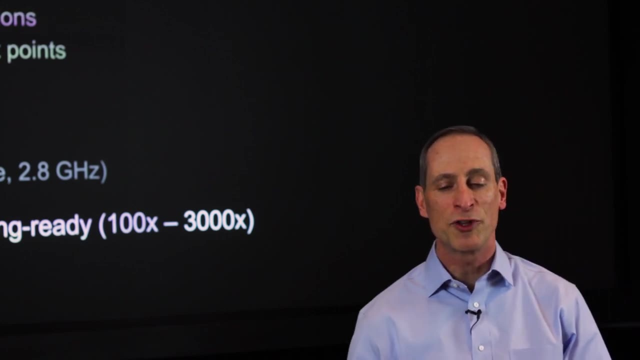 took advantage of the multiple cores on that machine. However, at some point it's very likely that this kind of problem is going to require cloud computing or some other high computing, high performance computing system, So the tools that we've chosen in this case had already been demonstrated in that. 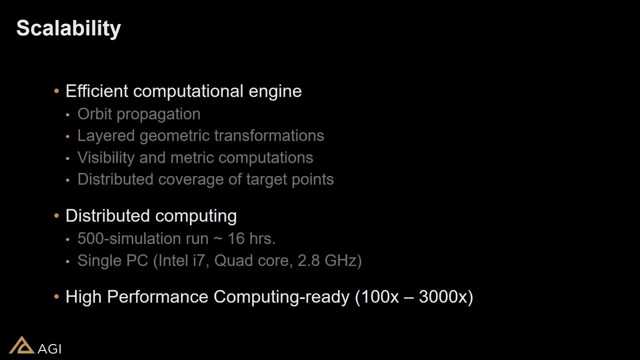 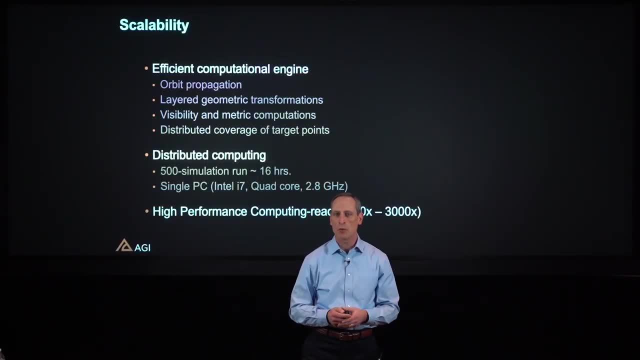 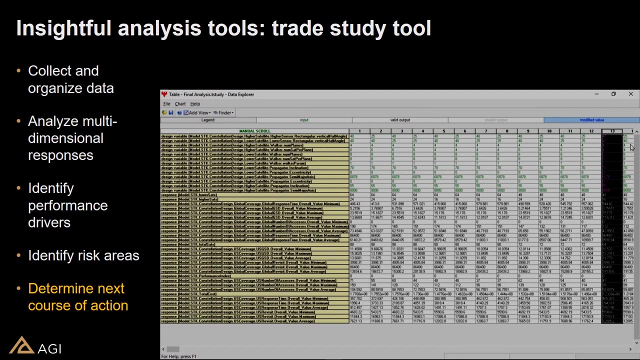 type of environment for highly scalable solutions. And then the final step in our process is now to take the results of that calculation and understand what happened and set ourselves up for the next iteration. So this is where we need to have a series of insightful analysis tools to help us look through this. 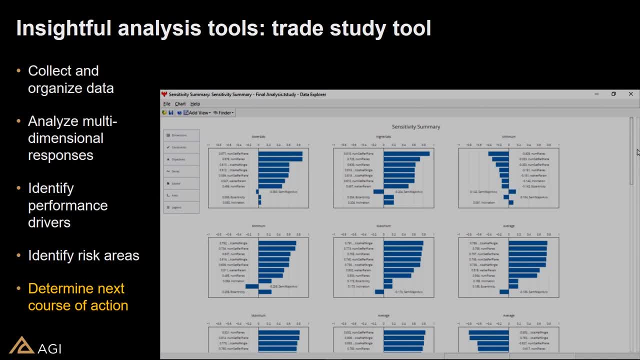 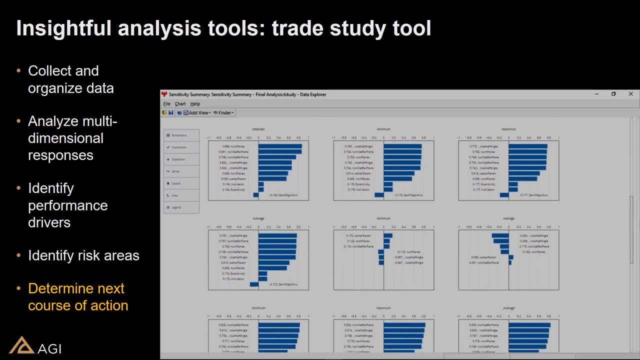 multi-dimensional data, and the fundamental things that are required are to ensure that the data is easily importable into the system and that we have the right kind of tools to analyze the data and look at different aspects of interest. So what you see here are a series of what are called tornado plots. 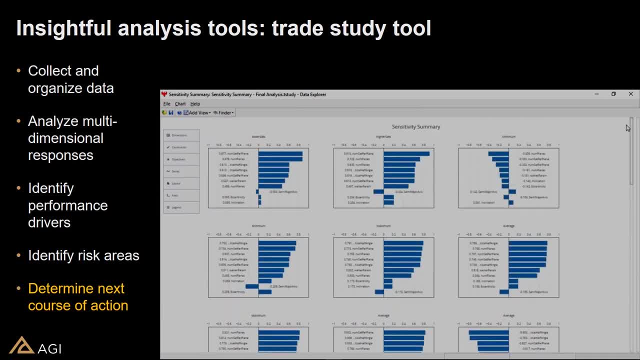 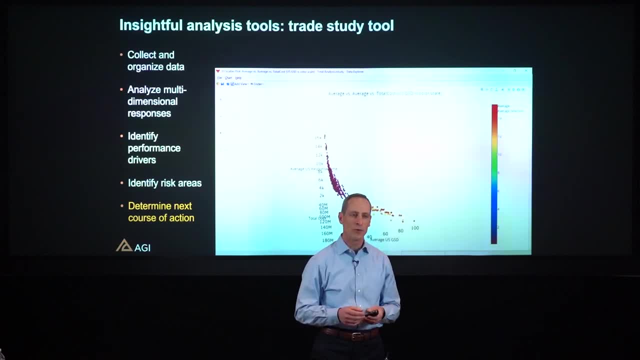 that, for each control parameter, look at the sensitivity of the various outputs. These help us identify risk areas, and there are a lot of techniques that are available to evaluate multi-dimensional data. So here you see a 3D graphical component that allows you to look at. 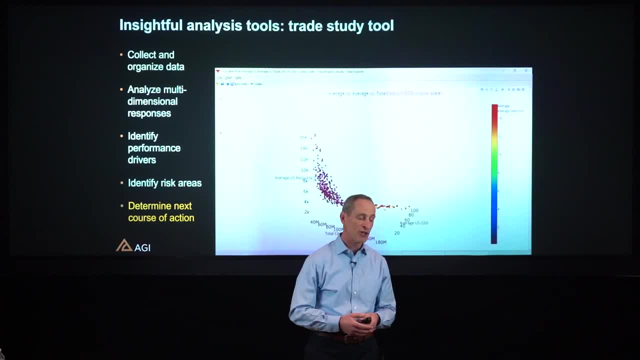 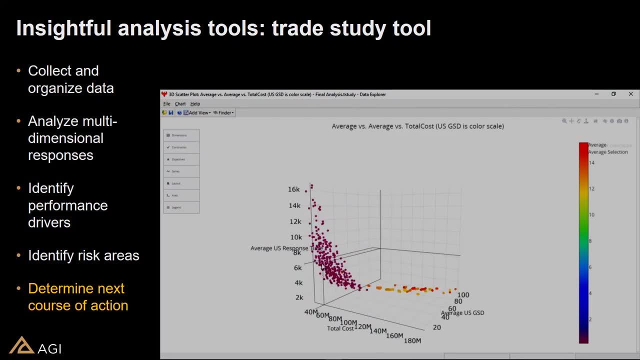 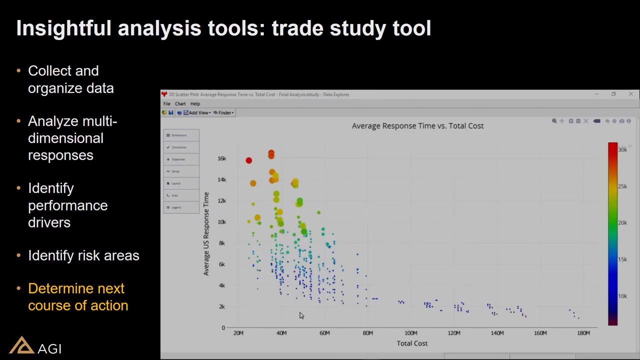 three-dimensional data, Different dimensions of data, to incorporate another dimension as a color code, and has useful attributes like the ability to individually evaluate data points within your data set and to be able to dig into each one of those, So you could actually spend days or weeks just going through some of the 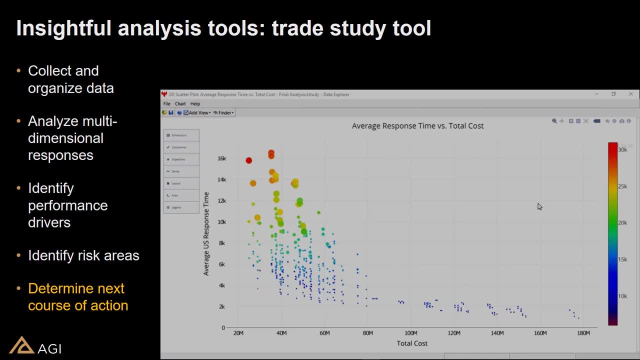 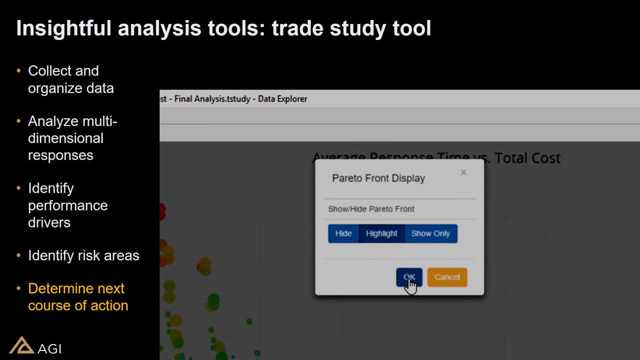 techniques available to do this. I just like to go through one here, which is one that I like to use, which is simply start with a scatter plot in a two-dimensional nature. So what we're looking at here is the average resolution in our high area. 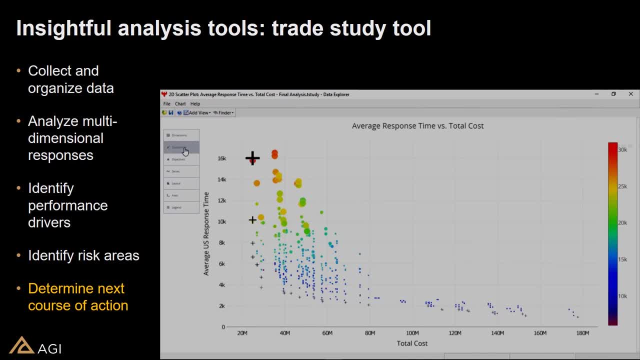 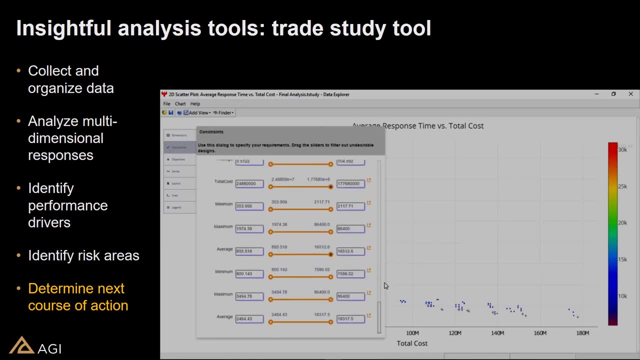 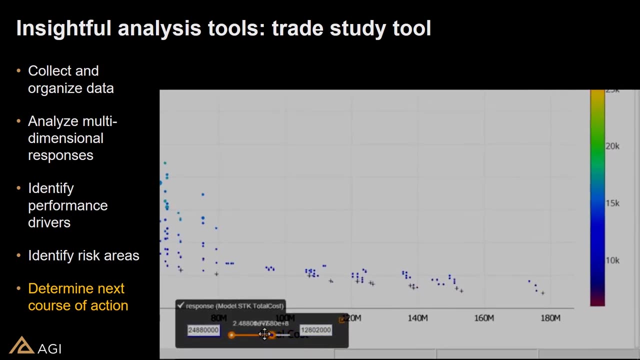 region of interest in the United States and cost along the bottom axis. And what we just showed is the creation of the Pareto front, The most important points, the highest effectivity points along the bottom. Now, frequently, with the multi-dimensional data, there will be aspects of your response parameters that 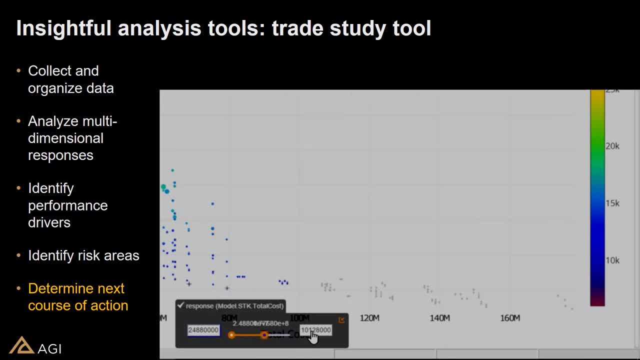 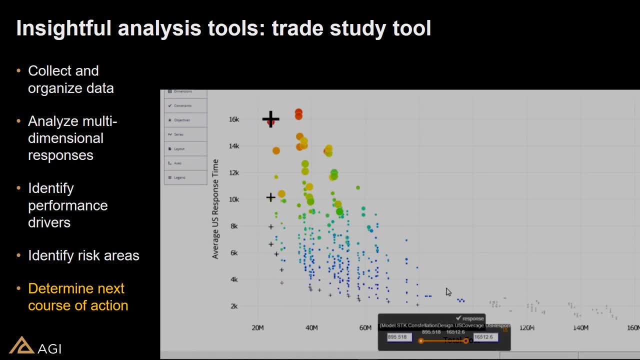 just simply aren't acceptable. So using features like this that allow you to go in and choose some of the most effective responses that you can get is called the use some of those other response parameters that aren't graphed here and simply take out unacceptable points, becomes a useful feature. So what you see 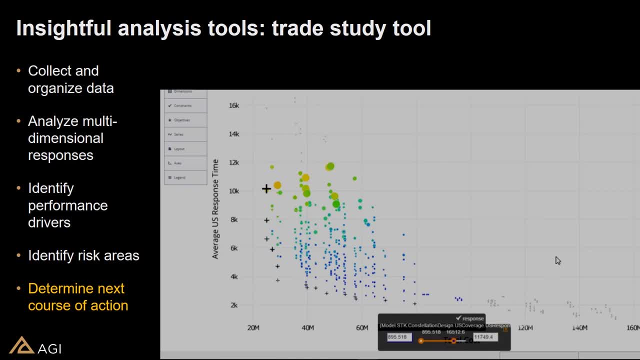 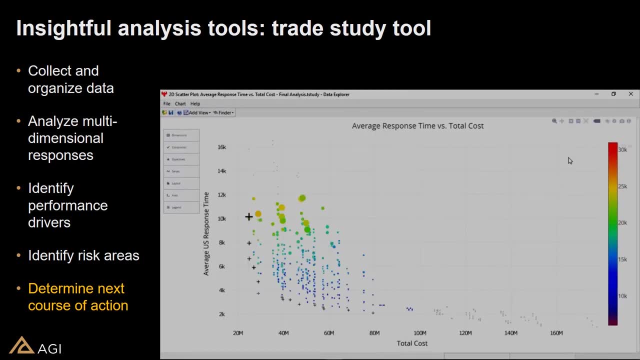 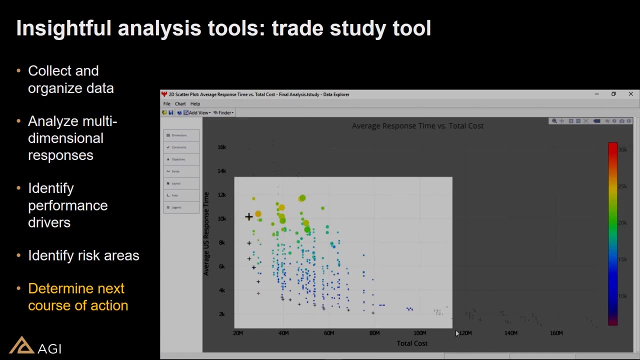 here is our filtering out points that are too expensive and others that are underperforming in other measures of effectiveness that we didn't include in the graph. Now that we've necked down our problem a little bit, we can zoom in and we can start identifying those areas that we want to focus in on for our next. 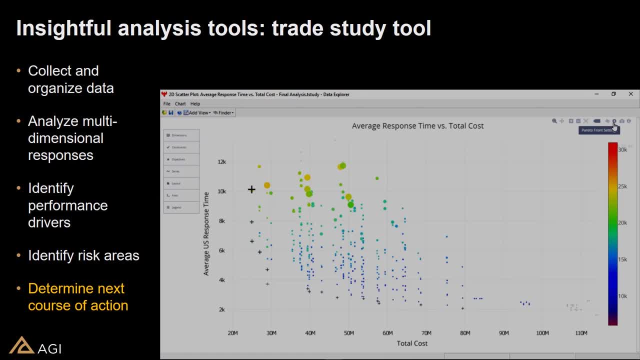 series of iterations. What we'll do now is we'll look at only those most important points. So I mentioned the Pareto front when we first set up those, the graph, and these are the points that are optimal along that bottom curve And if you go into any one. 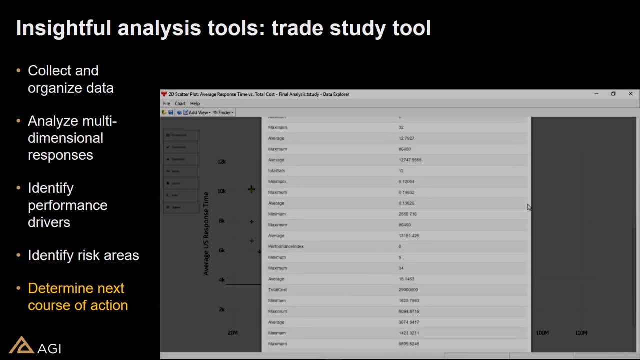 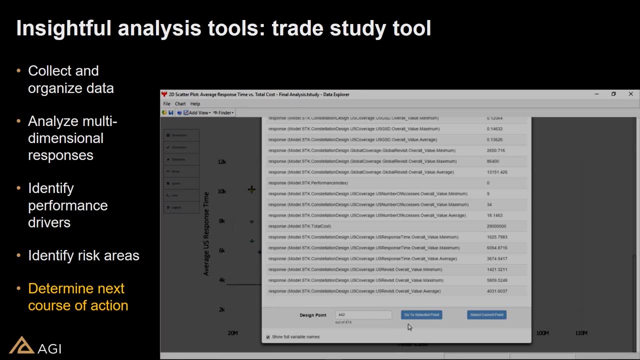 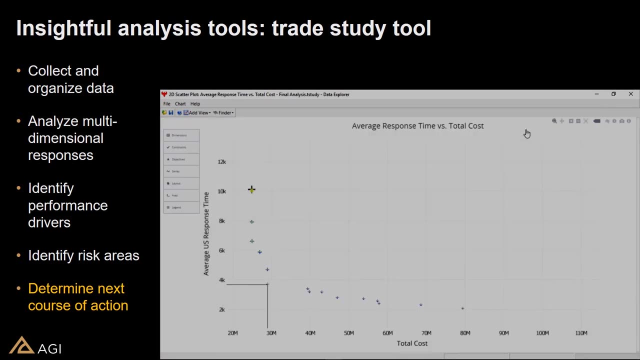 of those. you can pick the point that now becomes the center for your next iteration and your next trade study analysis and you can simply incorporate that back into your trade study tool as the starting point for your next trade study analysis. So again, the idea here is to take multidimensional data and to evaluate it. 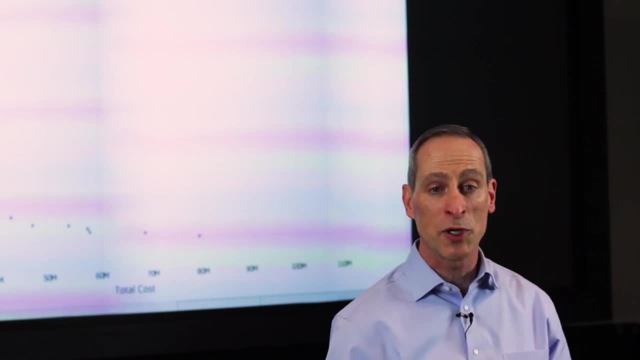 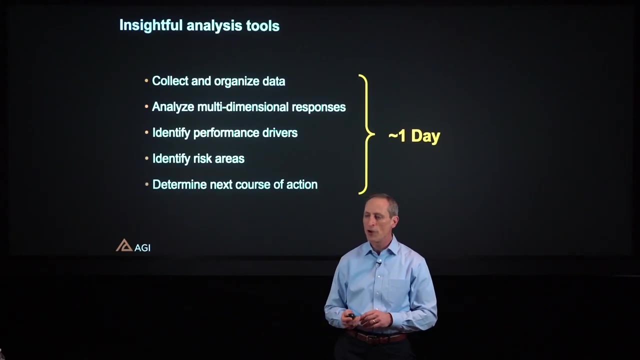 so that you can understand what happened, understand the relationship between the control parameters and understand where you should go next with and avoid areas of risk. So with that process it took us about a day to go through the collection analysis of the data and really the collection of the data took no time at. 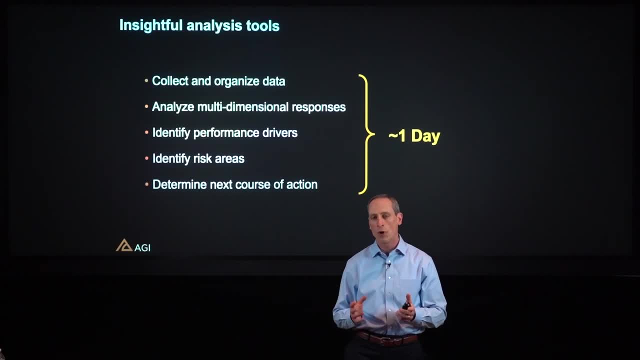 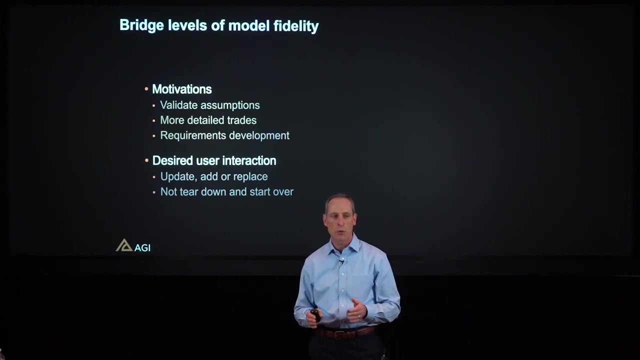 all because essentially, this is all one data framework. What took some time was the human analysis of the data and understanding which parameters we should plot against which others and interpreting what the data meant. So, essentially, in the span of less than a business week, we went through an entire cycle of that process. So what we'd like 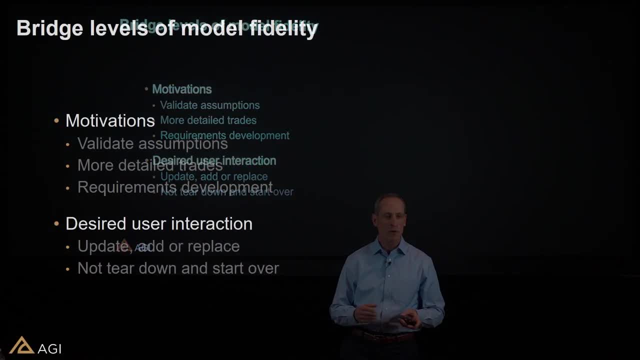 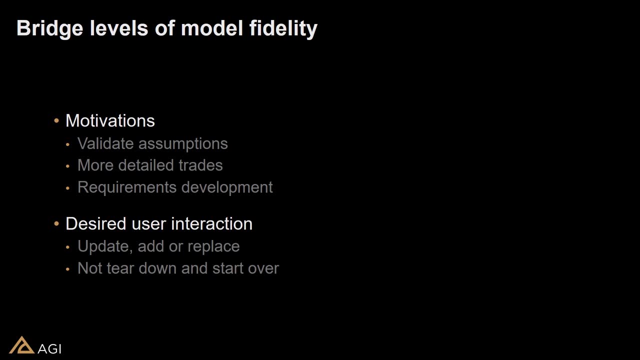 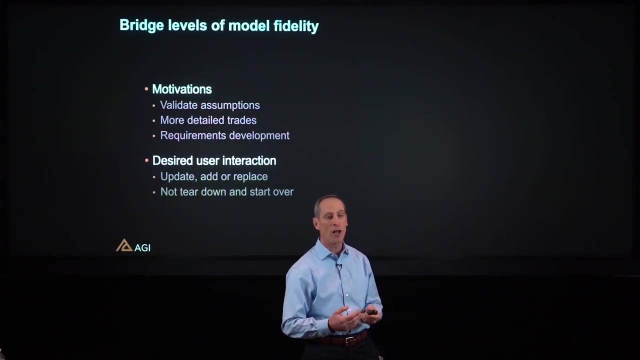 to do now is to look at what comes next, After we've been through this process and we've evaluated the first and second order conditions, how do we move on and identify the aspects that are more important as we bring in higher levels, of higher fidelity, or even move beyond the architecture design phase and start? 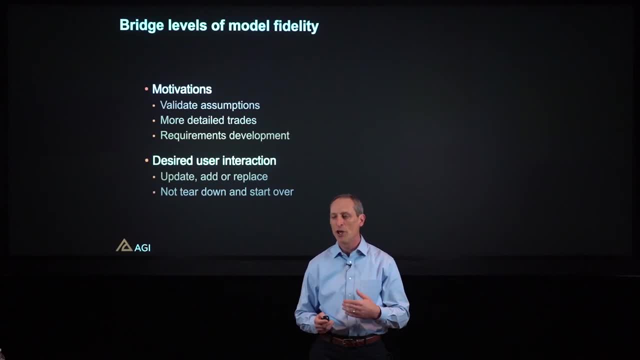 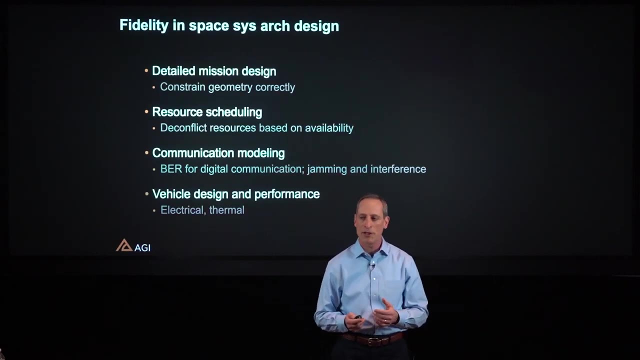 driving requirements for the systems engineering process. So that's where we want to bring in models of different fidelities. So I'm going to quickly go through some of the models that can be easily incorporated into this mission model and we'll talk about some of the factors that they bring to bear in this. 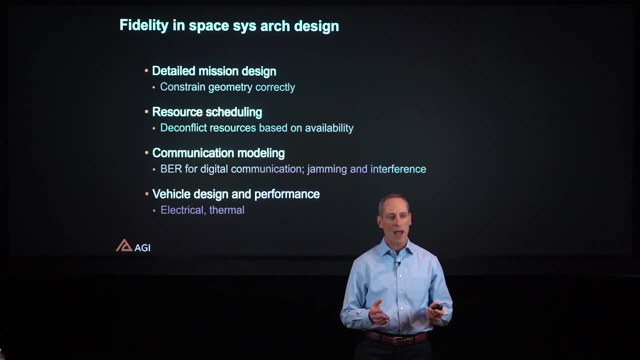 process. So, first of all, I talked about one of the measures of mission effectiveness being the system response time, and I like to use the example that we had in our reference case, because it makes some good engineering assumptions But essentially, at some point, you want to get beyond that and incorporate more detailed. 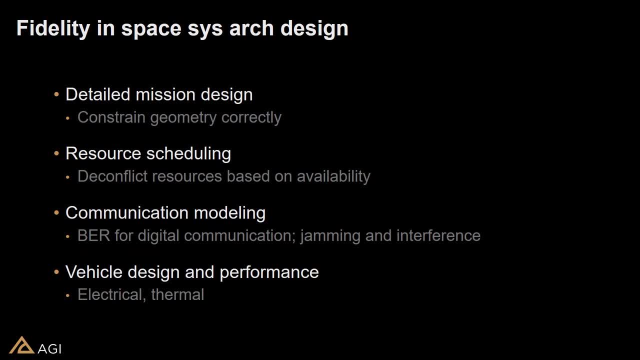 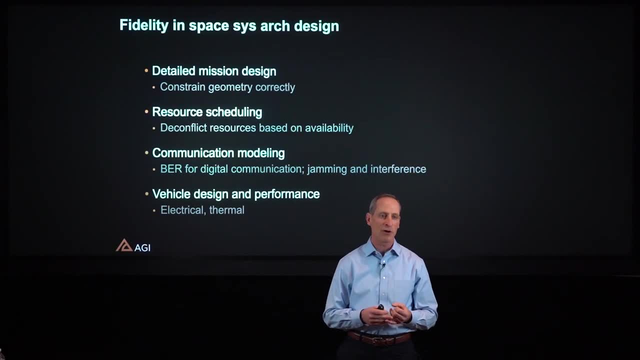 descriptions for how the system interoperates and how your measures of effectiveness are generated. So it's important to have tools that allow you to find those very accurately, And all measures of mission effectiveness are composed of four things: Position, where the target is, for example, the direction. 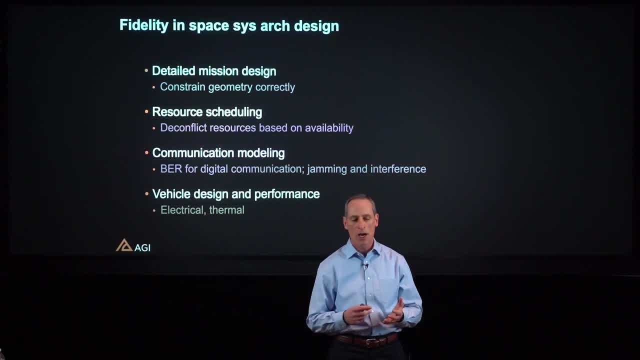 the direction that I'm looking, the direction of a sun angle, the time at which things occur and specific calculated values. So you need a tool that calculates all four of those things and lets you combine them easily. in order that you can do something like that- Another area that we'll need to look into- 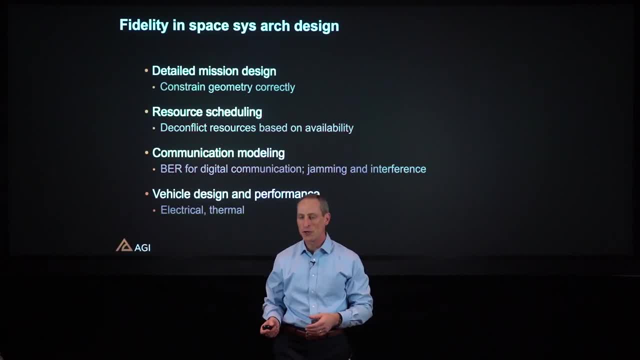 a little more closely is the availability of resource or resources or resource scheduling. So commonly in first-order analysis we assume resources are available that we aren't going to have constraints. That's almost never the case, So being able to incorporate a scheduling and a tasking optimization 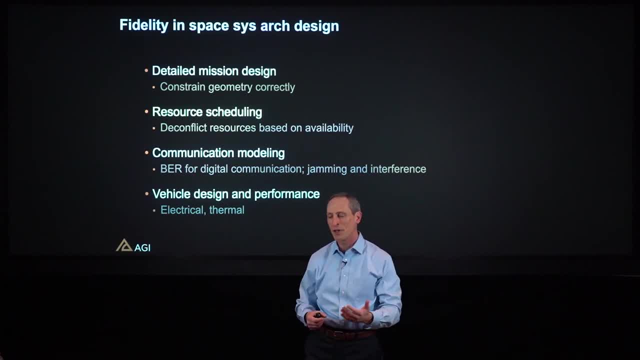 engine as part of this is critical. That's one of the tools and one of the model capabilities that ought to be able to fit in in the incorporation of higher levels of detail into these mission models. Same thing for communications modeling at different levels of fidelity. all the 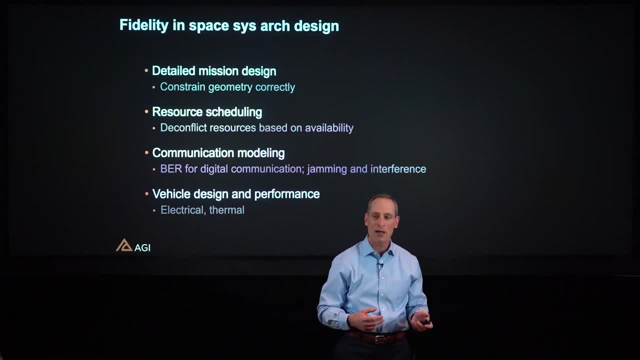 way down to the design and the operation of the antenna- if you're using phased arrays- the incorporation of beam forming algorithms and also the vehicle performance. So we gave no consideration in our first-order analysis to the vehicle itself. We created it and considered it only as an orbit, but all. 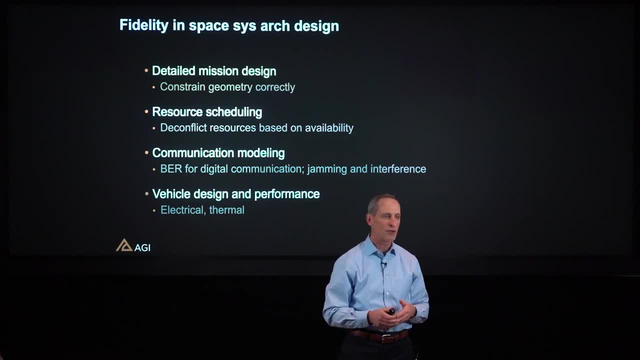 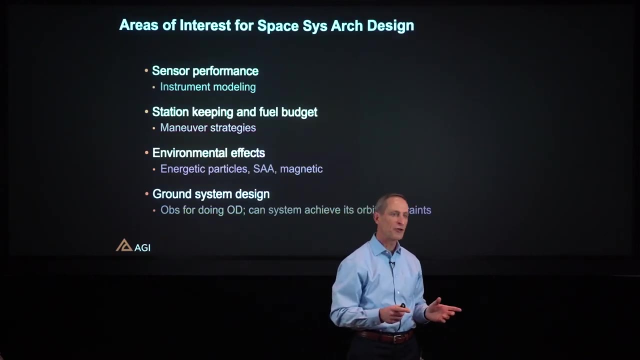 of the key subsystems on the satellite system ought to be incorporated to evaluate things like the power collection and what the driving requirements are going to be as you consider moving from the constellation design into the vehicle design. We talked about the sensor mostly from a geometric and resolution perspective, but also the fundamental. 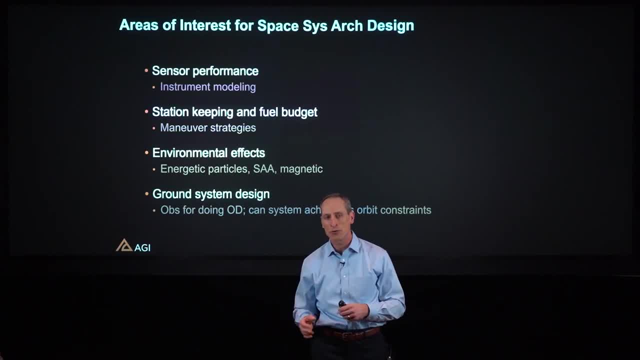 physics of the sensor are important. And again, remember what we're trying to do here. We're trying to consider missions that may not be the initial primary mission. So if, for example, you have a visible imaging sensor intended for use for ground surveillance and all of a, 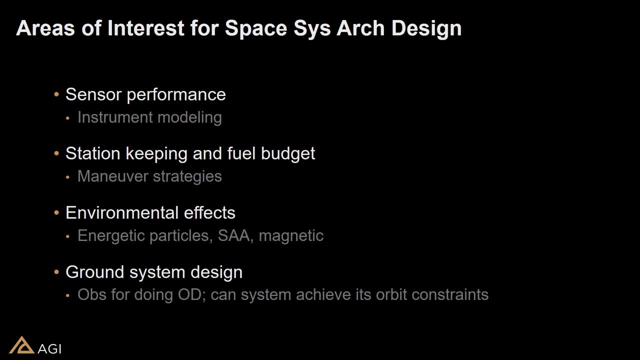 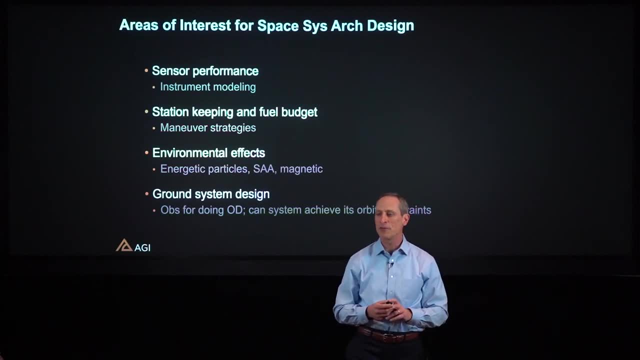 sudden you want to reapply your system to do space surveillance. having a physics-based simulation of your sensor system is absolutely critical in this level of analysis. Same applies for the ground system. Again, we didn't give much consideration to the ground system in our first-order design. but 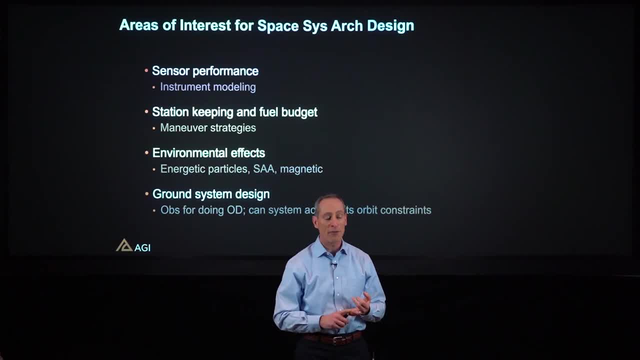 looking at the number of ground stations that are required, the kind of hardware that's going to be needed in order to provide the orbital estimation. fidelity are key components that have to be incorporated into this mission analysis at some point. Environmental effects, as you consider the lifetime of your system, become very important, and then the 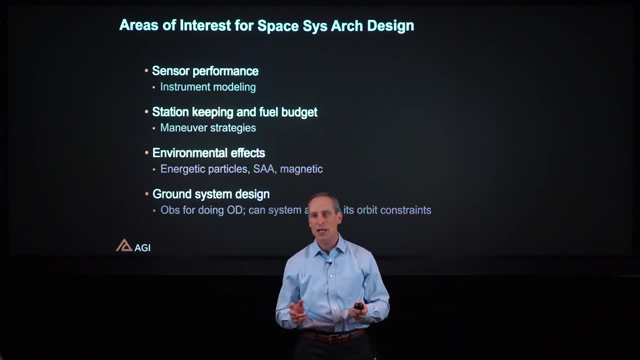 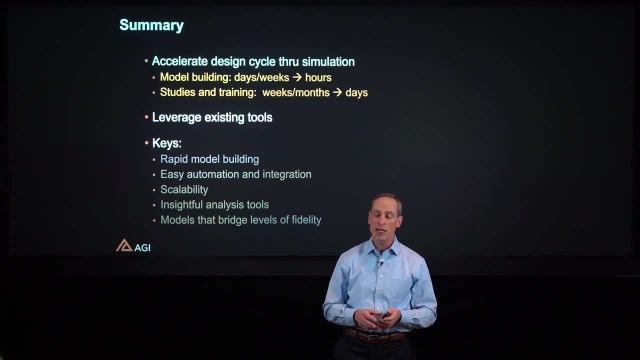 ground system design as well. So these are all aspects that can be incorporated into this kind of model that we illustrated in the first-order analysis. So, in summary, what we talked about is a technique to perform automated space system architecture design, particularly in the context of what we're seeing in the 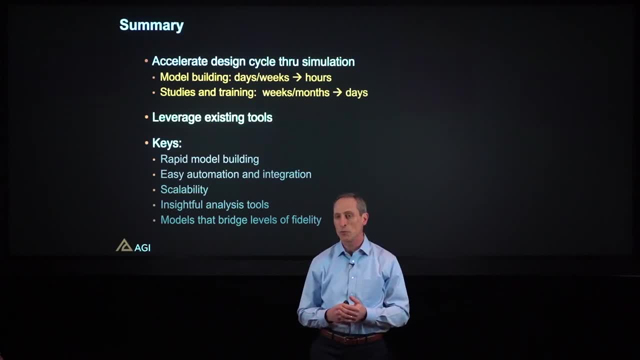 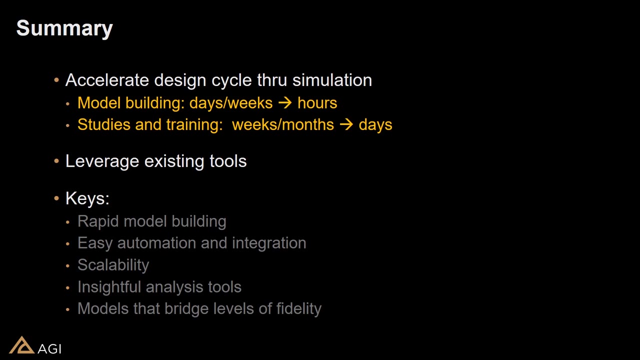 community right now, which is to dramatically accelerate the speed with which we conduct these kinds of studies and convert times that we're used to measuring in months and weeks down to days. This is readily accomplished by taking advantage of tools that are already in place and optimized to 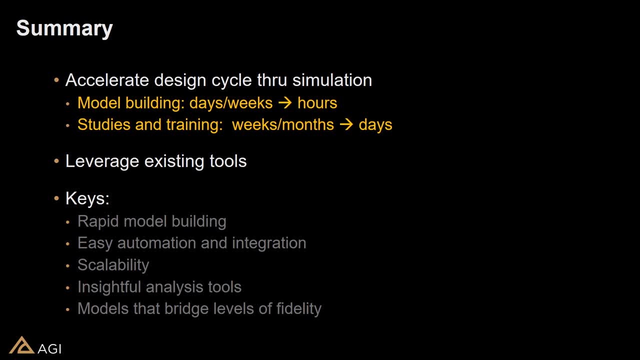 perform this kind of function And the five key areas that we identified over the years of our research? are these five key areas that we identified over the years of our research? are these five key areas that we identified over the years of our research? are being involved in this? are being able to? 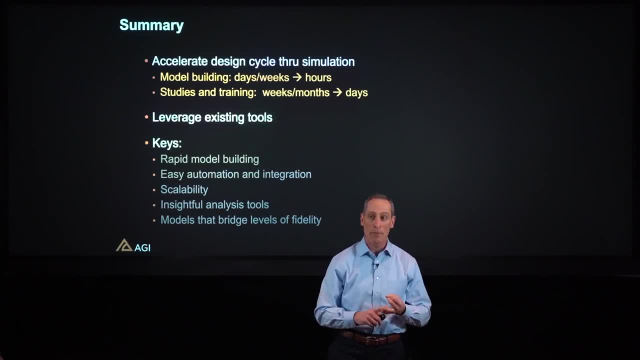 build those models very rapidly. instrument and automate those models. ensure that the execution of the simulations are very scalable. ensure that we have good, insightful analysis tools so we can understand the results that the models produce. and ensure that we can transition from each phase of the. 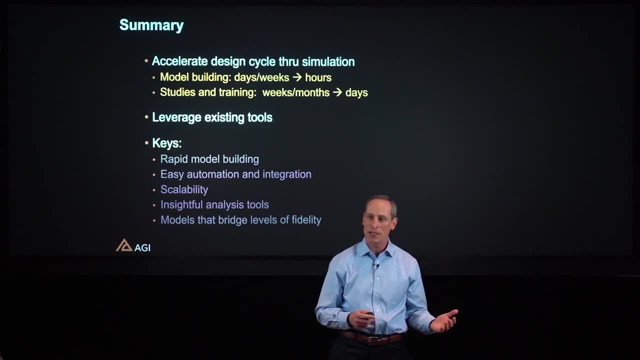 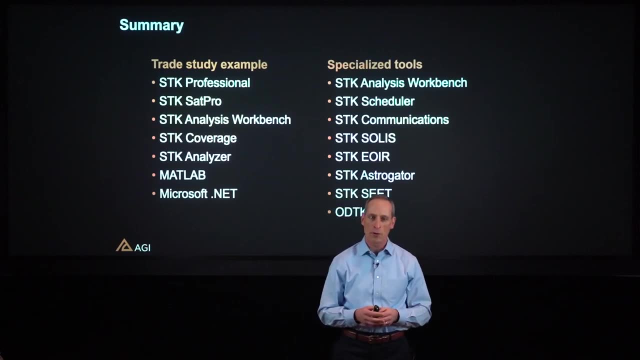 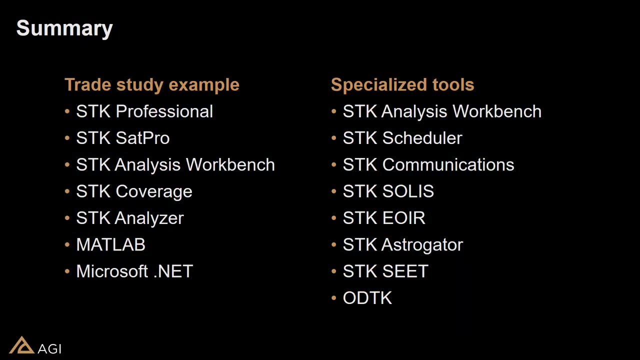 process by adding models of higher and higher fidelity without having to go back and rebuild the fundamental mission model. So when we did this, clearly we are going to use our tools. so these are some of the tools that were used in the first part of the analysis. for the trade study, we used SDK. 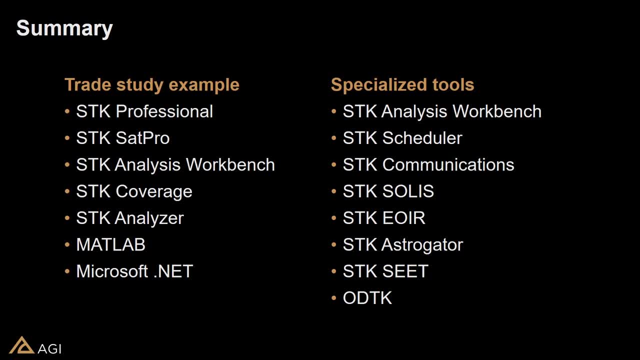 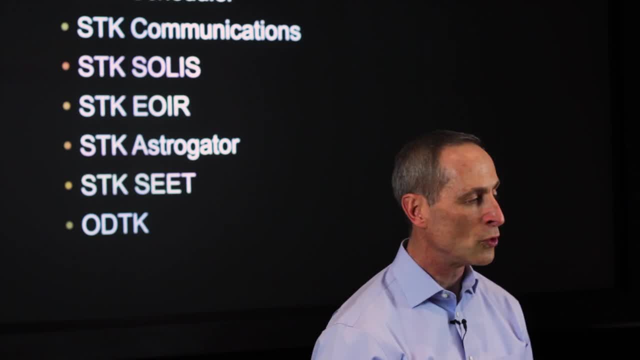 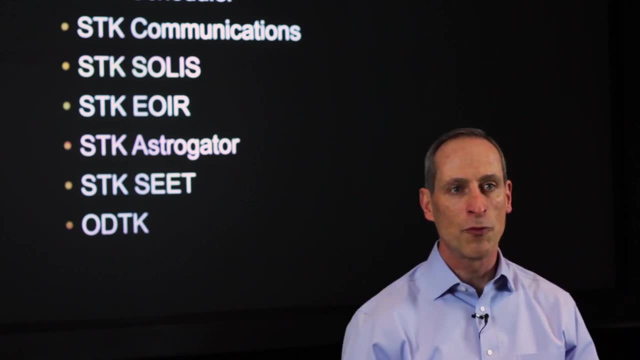 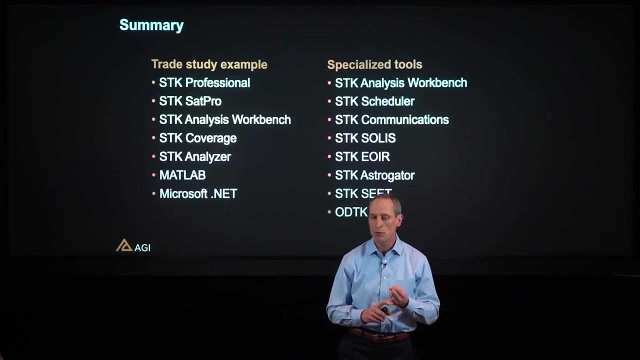 professional SAP pro for the orbit propagation, the SDK analysis workbench, which helped us define some of the key measures of mission effectiveness, the coverage tool that allows to rapidly grid ground-based points of interest, SDK analyzer for the automated trade study, and then we incorporated other third-party tools. we also did the trade study automation using MATLAB, which we